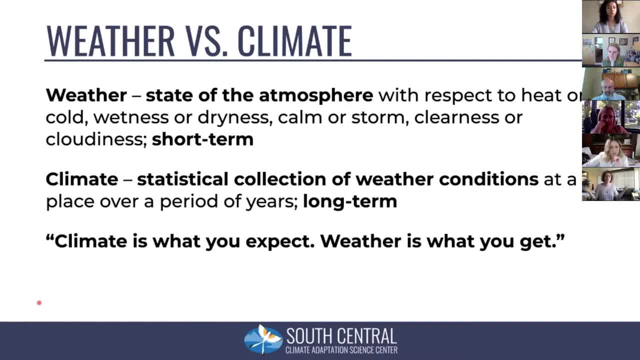 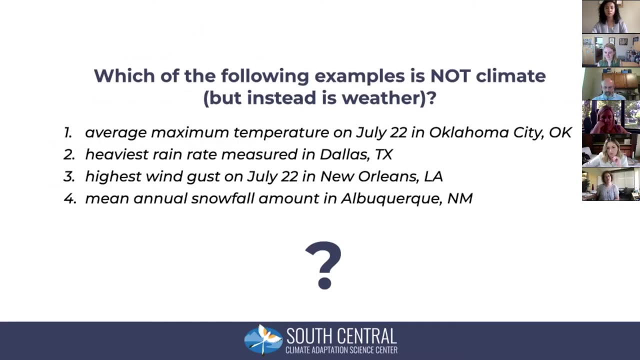 that place and in that season. we compare it with what's happened at other times in that place, and so climate gives us a context. it's long-term and in some cases you may have heard the phrase climate is what you expect and weather is what you get. so we're gonna start our first poll question. if you will read these: 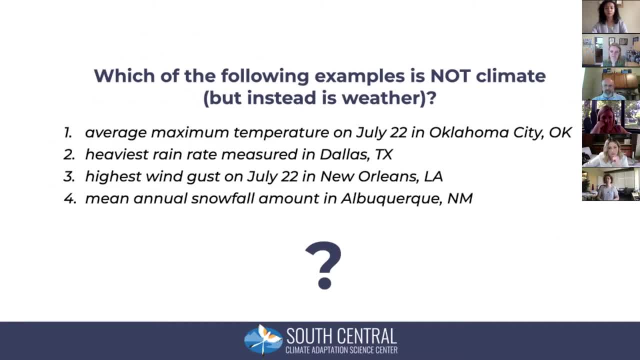 examples and pick out the one that is not climate-friendly, and we have a couple more experimentation on climate. you're looking for the weather example. Okay, we have about twelve responses so far. I'll wait another few seconds. Okay, so how many impressions we get? satu response so far. wait another few seconds. 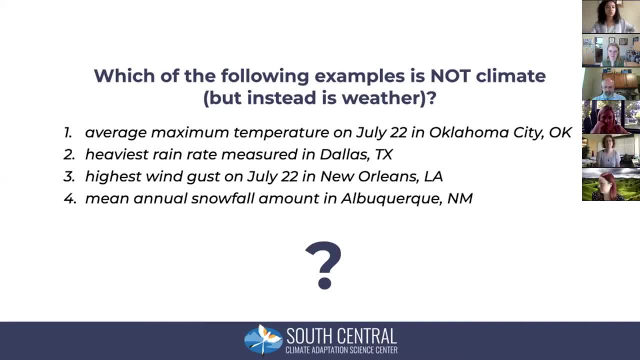 for you to respond. all right, so we'll end the poll and share the results and excellent, good job. so the highest wind gust on a particular day in a particular location, so this is a very specific event that occurred. if we compared that to other wind gusts on other days to see if, if it was the highest that 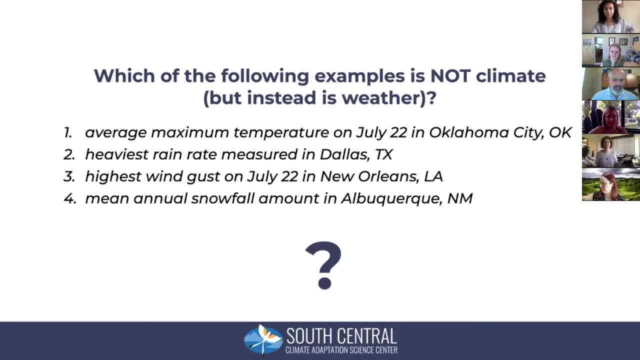 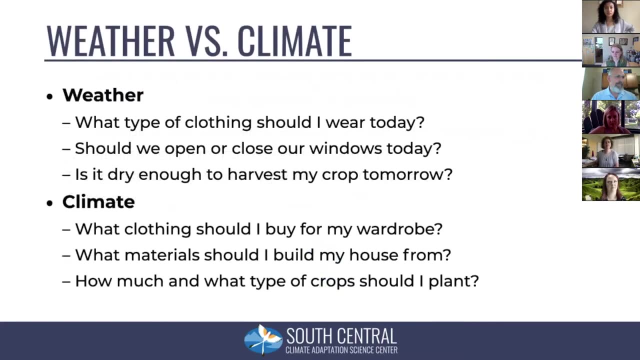 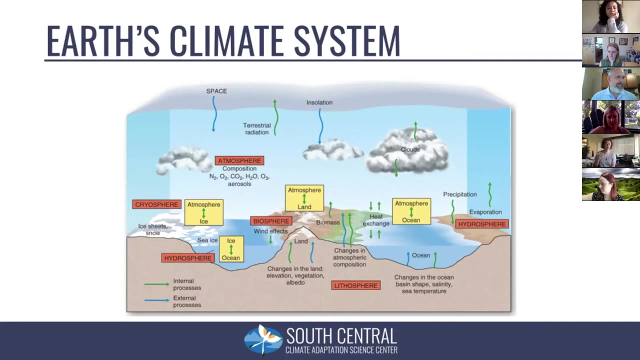 occurred ever in New Orleans, then we would be talking about climate, but in this case we're just talking about weather. so let me close that. so this, This is our climate system. So a lot of times when we talk about climate change, we hear about the average global surface. 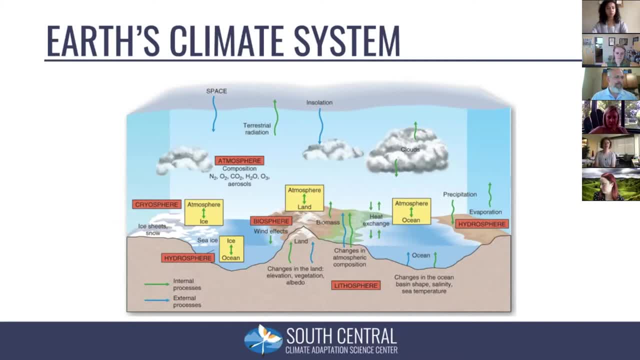 temperature and how that's changing over decades and centuries. That's only one element of our climate system. The climate system interacts in both the water, the land, the vegetation and the atmosphere. It interacts with each other. So when something changes on a global scale, like our temperature, then that's going to 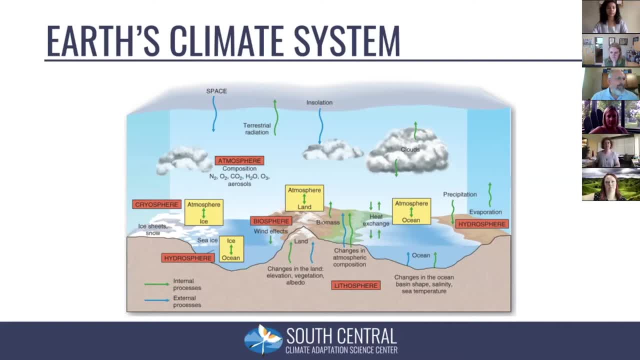 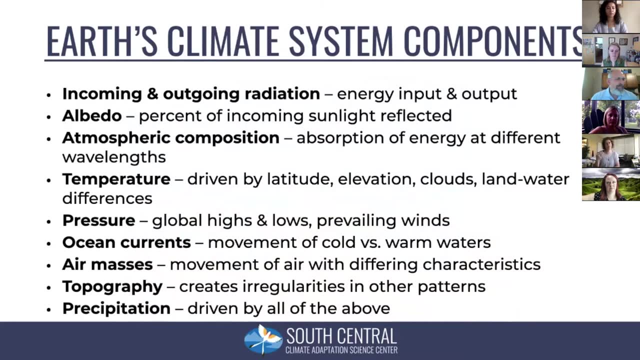 interact with all the other parts of the system. So if we look at some of the big components of our Earth, This is the list of them. You probably have heard these terms before, with maybe the exception of albedo, So that's not a really common term, but albedo is simply the percentage of incoming sunlight. 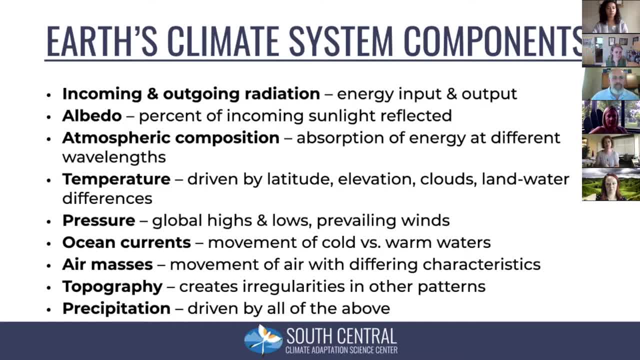 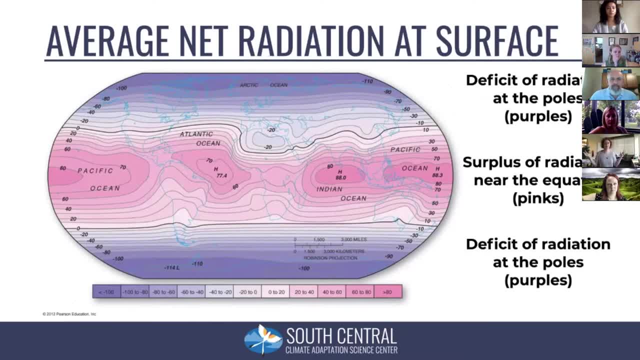 that we get reflected off of our Earth. So let me walk you through each of these and why they're important. So this is, This is our climate system, regardless of climate change. This is our climate system at its heart, And it really starts with this average net radiation at the surface. 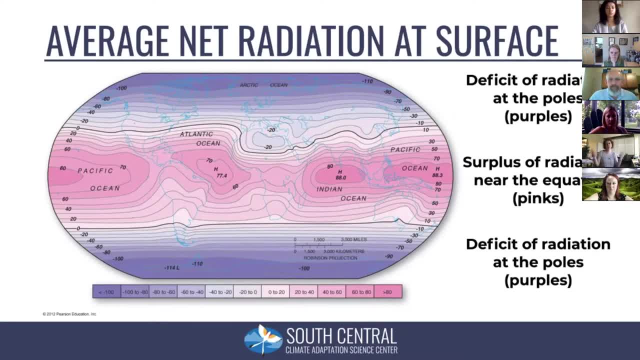 So that sounds complicated, but basically what it is is it's just a bank book of balances. So you have incoming solar radiation, You add that at the surface, You have that reflection of solar radiation that I mentioned through the albedo. So we deduct that from the surface. 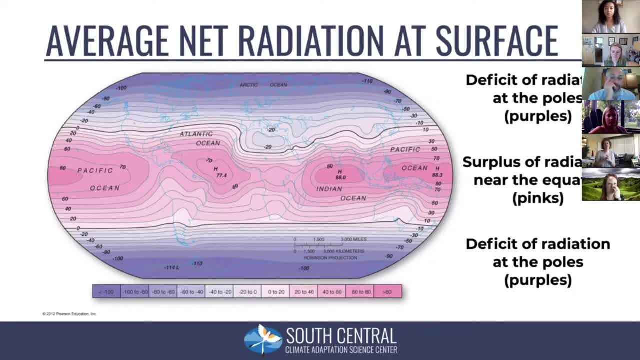 We have incoming radiation from our atmosphere, So that's at a different wavelength than the sunlight And that's added at the surface, And then we have the removal of some of that energy And that it Blue, Mesozoic. Both of that is radioactivity. 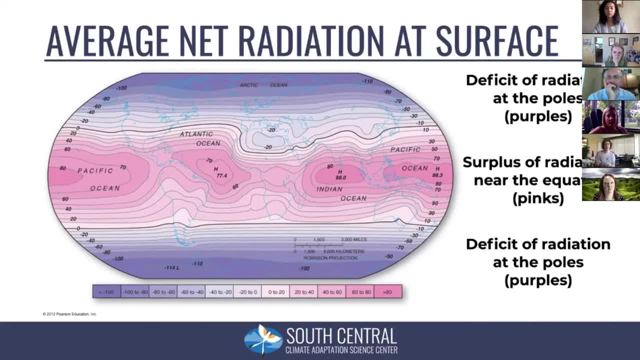 Right of that what we call long wave radiation from the surface, And we deduct that from the equation. So we add two components and we subtract two components. that gives us our net radiation. The solar energy that we have into our system is primarily at the wavelengths of sunlight. 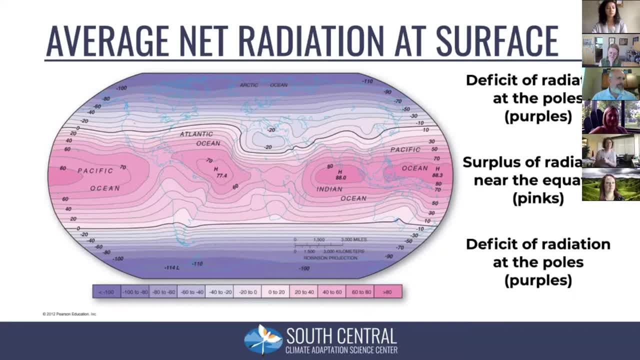 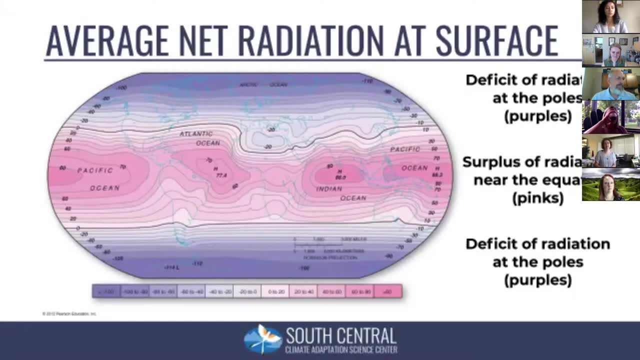 or well, of course it's at the wavelength of sunlight, It's at the wavelengths of visible radiation and ultraviolet, and then the radiation that we talk about, that interacts within our atmosphere and leaves our earth, is in the infrared. So we have different wavelengths of radiation. 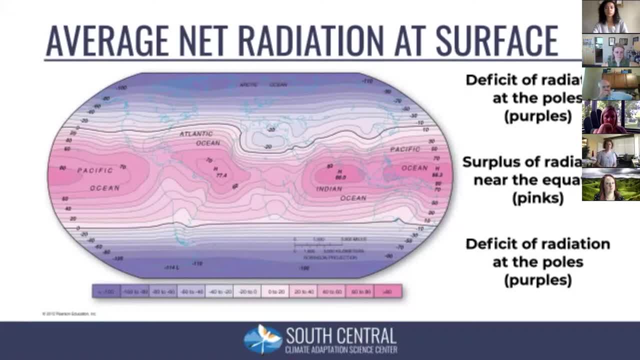 as a result of their sources. So this average net radiation. what you can see is that there is a surplus near the equator. So in the tropics and in the subtropics we get a surplus of net radiation, And then in the mid latitudes and the poles. 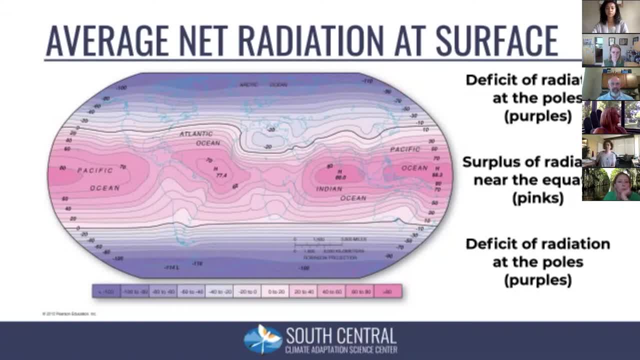 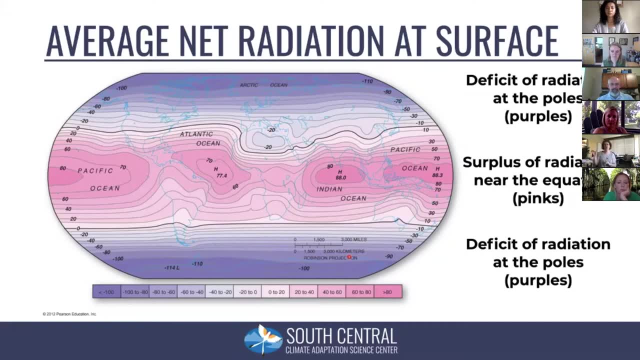 we have a deficit of net radiation, So this means more energy at near the equator, a deficit at the poles, and just like that you try to do with your bank book. If you go in one account in deficit, you got to. 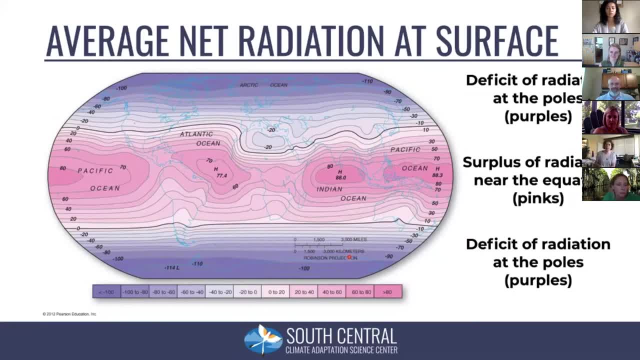 try to move some money to that account so that you can get it in balance. Our entire earth climate system is trying to do that. It's trying to move that excess energy from the tropics and subtropics toward the mid-latitudes and the poles. 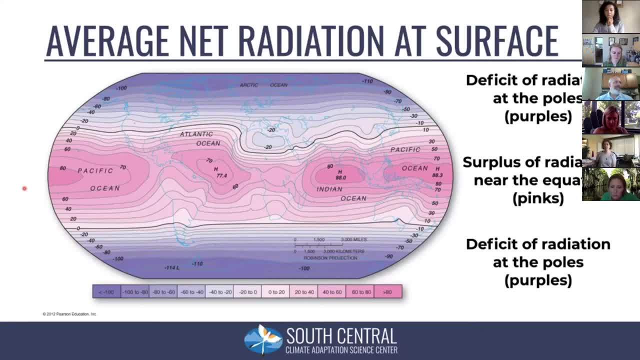 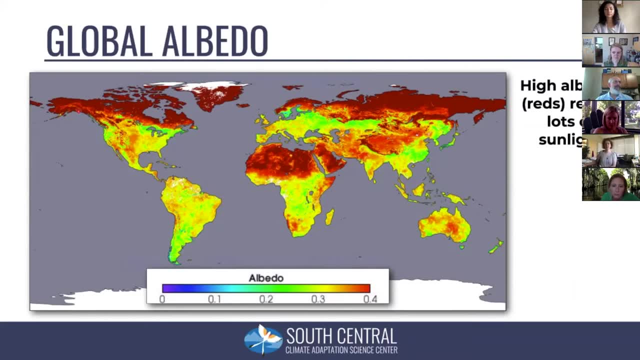 So that's our major driver. So part of that, as I mentioned, is related to this global albedo. So this is the reflectivity of the surface and it really relies on essentially what color that surface is. So areas that are very white or light in color, like you would see in these higher latitudes where we 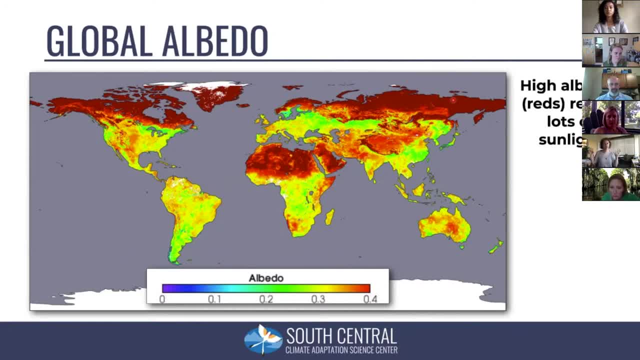 have lots of snow and ice are going to reflect most of the incoming solar radiation. Surfaces like these desert regions in North Africa and in the Middle East are also very light in color. They're going to reflect most of the radiation And one of the reasons why. 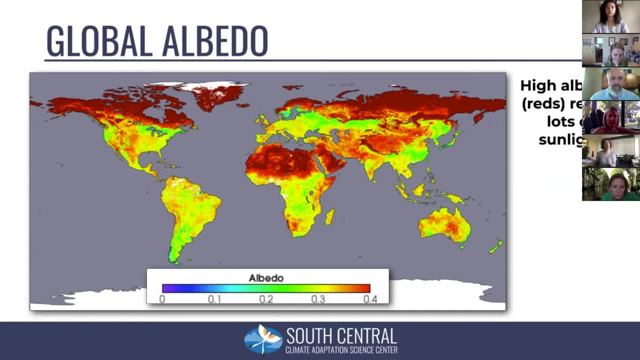 this is important is because in these snowy regions and icy regions, the surface starts getting darker, And when it gets darker, it starts absorbing more of that radiation and that warms the surface, And so one of the things that you'll see in global climate projections is that in the Arctic it is 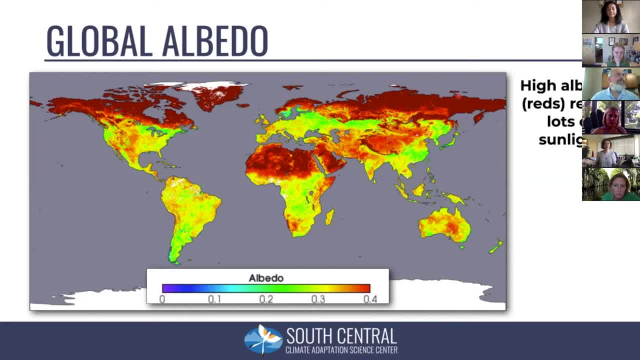 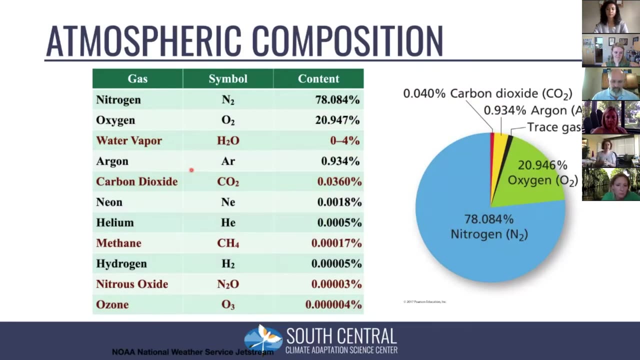 warming at essentially twice the rate of most other places on Earth, And so that's all a result of this change in that global albedo. Then we have the composition. So this is what are the all the different molecules that are in our Earth system. Most of it is nitrogen and oxygen, which is great for us to breathe. 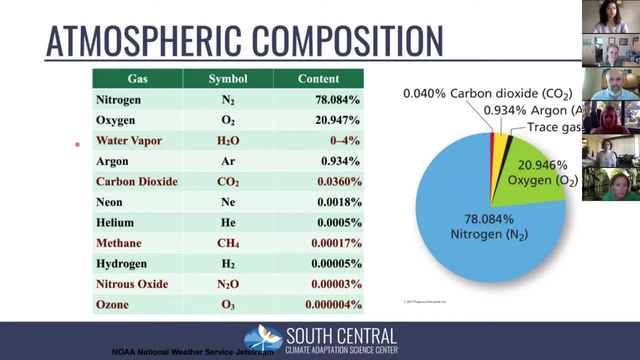 But we have some of these molecules in the system that we kind of refer to sometimes as trace gases. They're in very small quantities, like water vapor, carbon dioxide, methane, nitrous oxide, ozone. These are in small quantities but they have a great effect on our atmosphere, And so you can think of this. I. 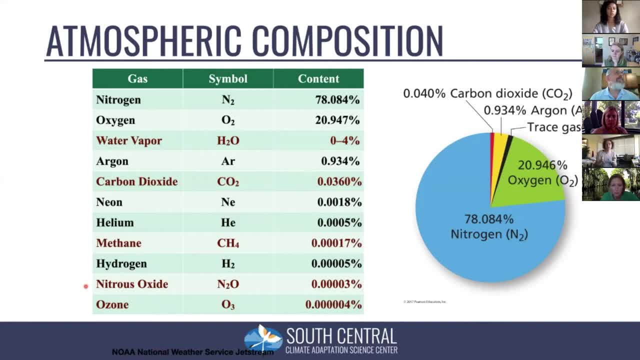 always tell my students in my class, if I give you a glass of water, maybe you're really, really thirsty. I give you a glass of water and I'm just going to drop a little bit of cyanide in that water- just a tad. There's not much in it, No worries, right? So they're likely not going to drink that. 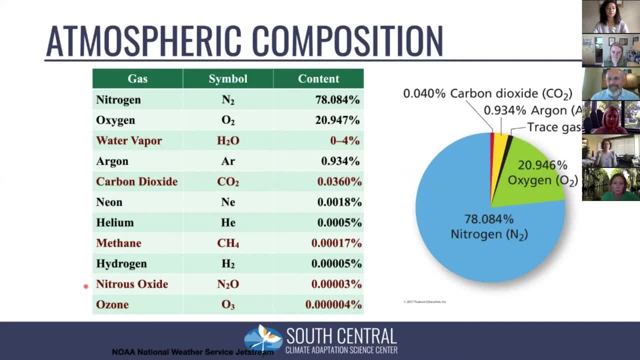 So, even though there's a small amount, it can have a really, really large impact, And so these gases that are highlighted in this dark red color might be a little bit hard to see, but the carbon dioxide, methane, nitrous oxide, ozone and water vapor, those we refer to together- 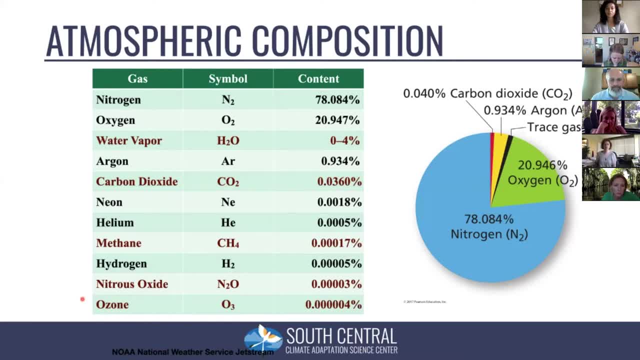 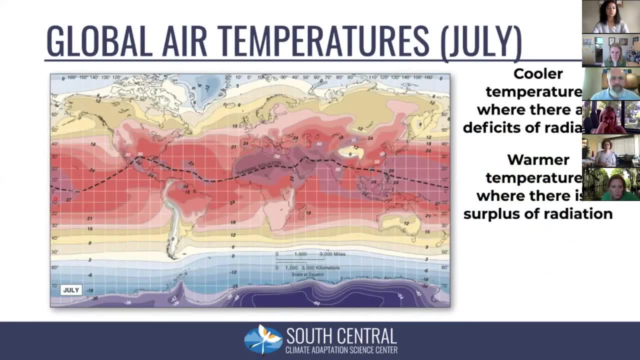 as greenhouse gases, And I'll show you later why these greenhouse gases are important. So another major element of our system is the global air temperatures. So these are air temperatures at the surface, either over land or ocean. And again, you see these. 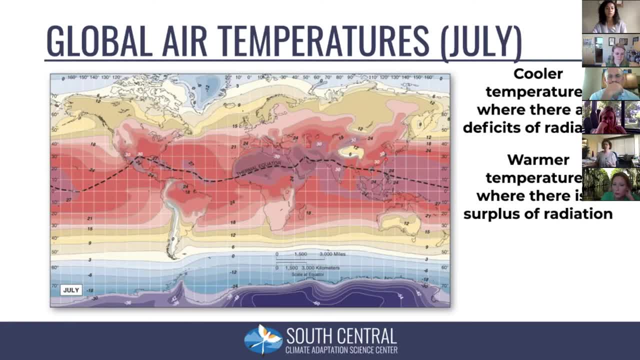 patterns. So these are the global air temperatures at the surface, either over land or ocean. And again you see these patterns. So these are the global air temperatures at the surface that result from this higher net radiation near the equator and the lower net radiation at the 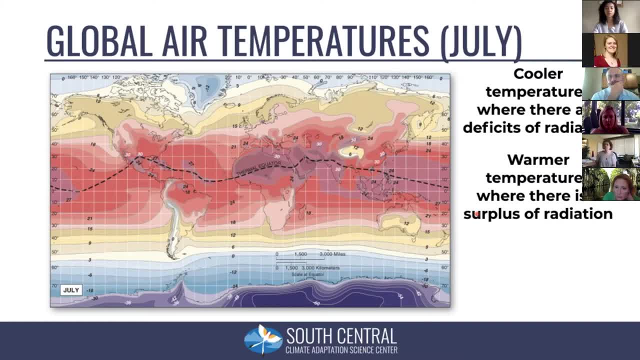 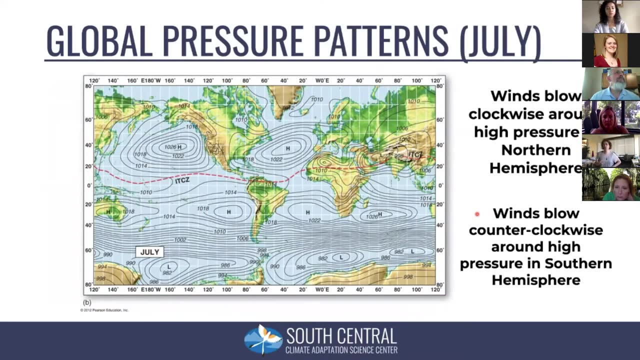 poles And depending on what season you're in- I'm showing July- one of the hemispheres warms up more and the other one cools down more, But those patterns are going to influence our climate. Then we have what we call the global pressure pattern, So you are used to. 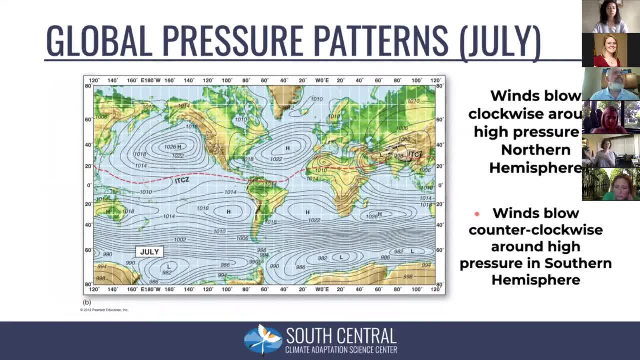 high pressure and low pressure systems moving by your location. That's kind of the weather version of it, what you see on TV. But the climate version is: if you average those patterns over time- the high and low pressure systems- you see these general patterns that occur. 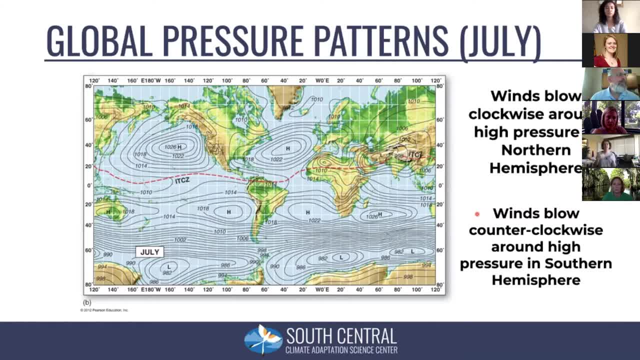 And they're caused by rising and sinking motion. That's a result again of that distribution of more energy and more energy, And so you see these patterns over time, And so you see these patterns of less energy at the equator and less energy at the poles, And so one of the things that we see with 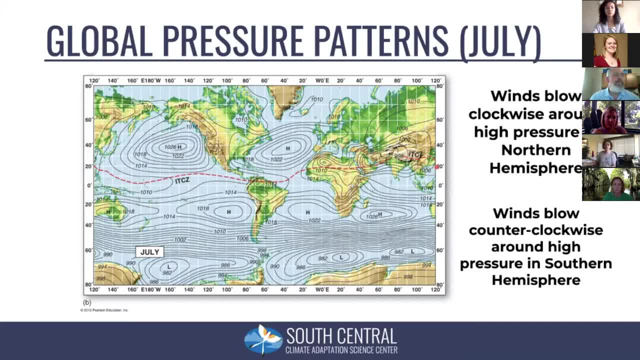 this is. we have generally rising motion along the equator, called the intertropical convergence zone, So that's a rainy region across our earth. Then we have sinking motion, generally about 30 degrees north and 30 degrees south of the equator. These end up being high pressure systems that predominantly 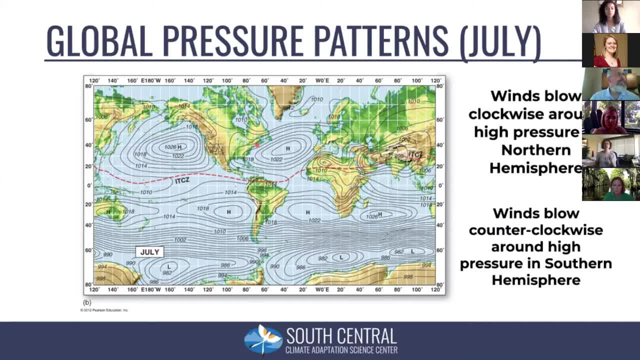 sit over our ocean basins. So in the northern hemisphere we have two main ocean basins, So we have two major high pressure systems, So the Pacific or Hawaiian high, the Bermuda or Azores high, And we have three major ocean basins in the southern hemisphere. So we see these three. 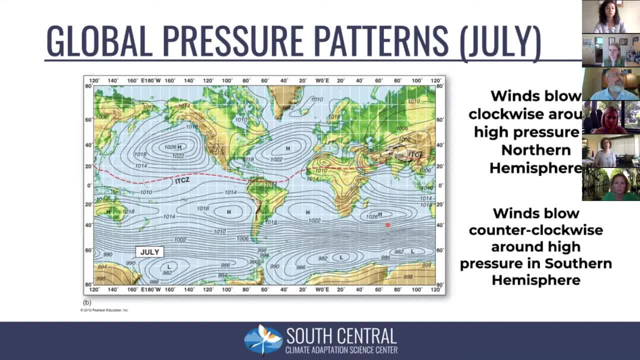 major high pressure systems And again, depending on what season it's in, they will move either northward or southward. And then we also see in this example these low pressure systems near the poles, So in the winter hemisphere, which is the southern hemisphere in this example. 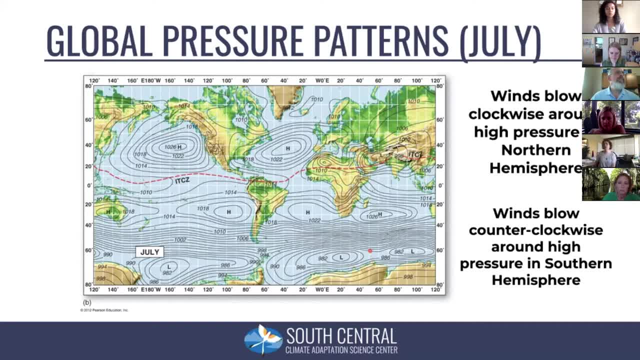 in the winter hemisphere we'll see these low pressure systems build. So if this were January, we would see the Aleutian low up here near Alaska and the Icelandic low build. And the important thing about these pressure systems is they forced the wind field. 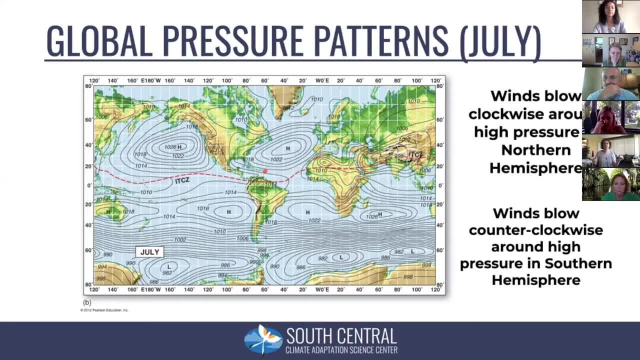 So winds don't exist without differences in pressure. So around high pressure systems the surface winds will circulate clockwise in the northern hemisphere and counterclockwise in the southern hemisphere, And so this is giving our surface winds motion That brings cool air from the north down toward the equator. 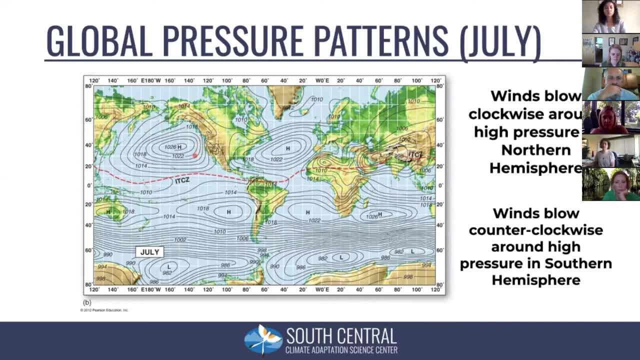 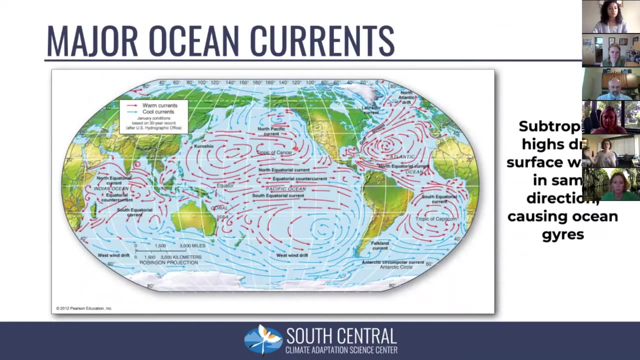 In this example of the high pressure system: warm air from the south toward the north. This is essentially our air conditioning system. This is what's distributing that energy from the equator toward the poles And also what those high pressure systems- these high pressure systems don't need the Springs- have to do with those high pressure systems. 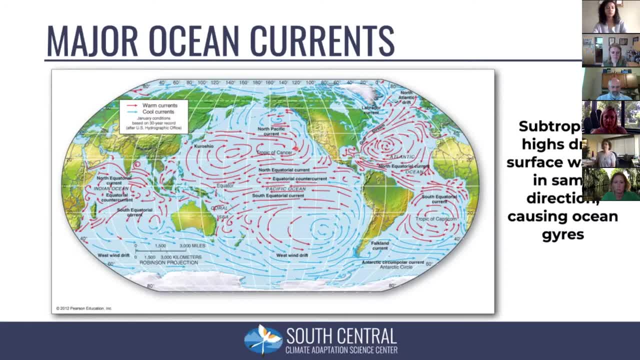 because of the region, And one thing that these high pressure systems do is because of those wind fields at the surface, they're dragging the surface ocean with it And that gives us our major surface ocean currents across the planet, And so you'll see that these ocean currents are going in the same direction as 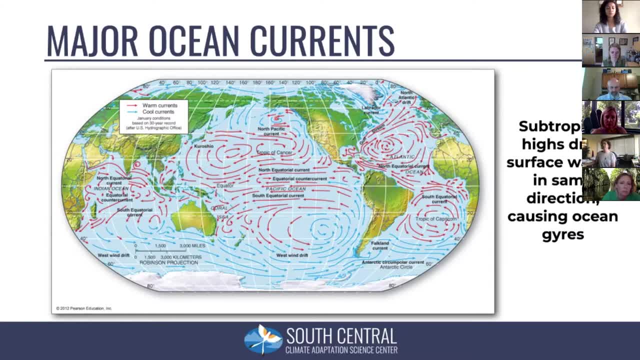 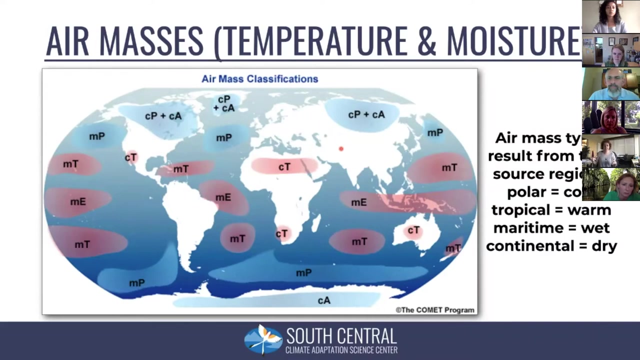 those large scale high pressure systems- again those high-pressure systems. and cold water to the south, again, redistributing that energy, moving that around. That's the fundamental way that our climate system gets in balance. So any changes to those systems. 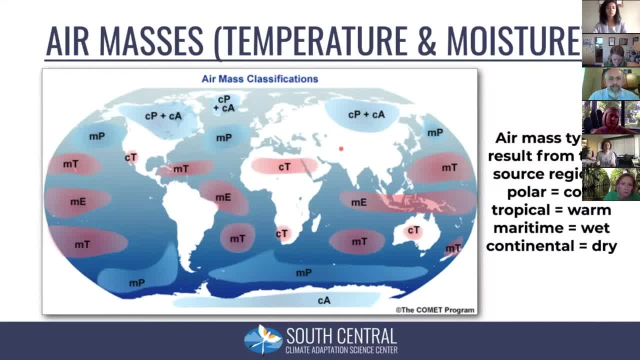 those high-pressure systems, those low-pressure systems. any climatological change to that is gonna affect the entire planet, not just right where that high-pressure system might be. So those systems, as I said, are moving bodies of air and we refer to these as air masses. 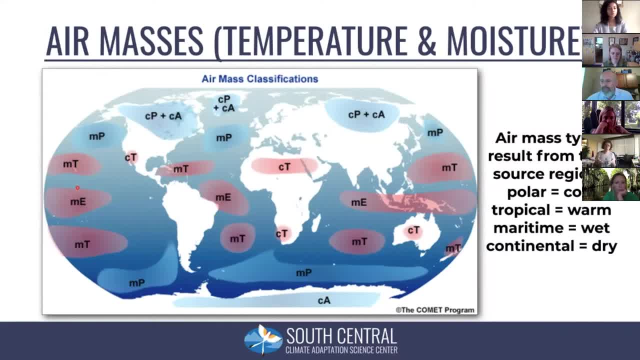 These air masses kind of sit for a while at a place and then they're moved by these wind systems, the high and low-pressure systems, And so the characteristics that they gather are based on where they sit for a while. So those that sit over the oceans we call maritime systems. 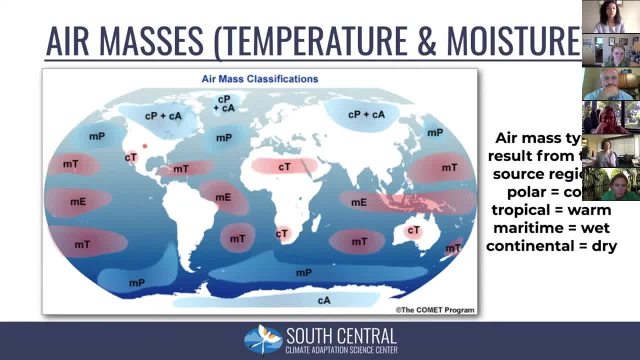 They have lots of moisture in them. Those that sit for a while over the land masses we refer to as continental air masses, Those are typically dry. The ones that are near the equator we refer to as tropical, So they gather a lot of heat. 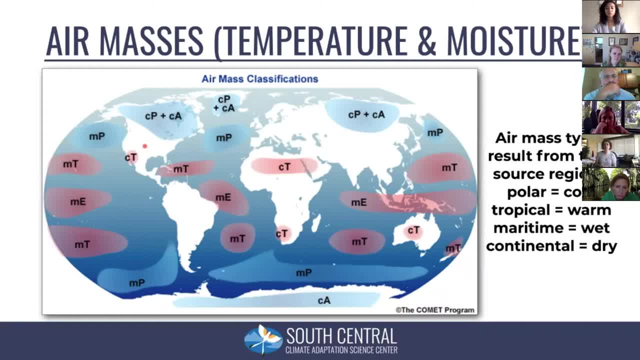 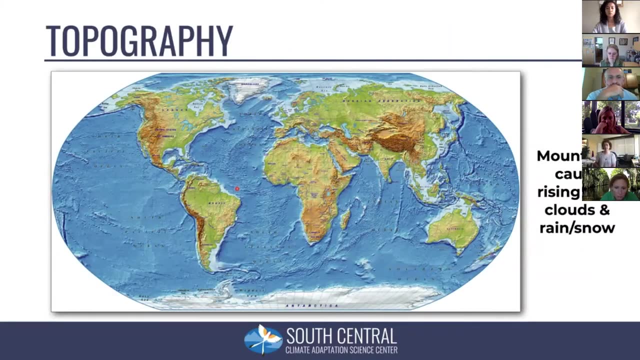 And the ones near the poles we refer to as polar Or Arctic, and they're gonna be cold. So those as we move those around, that gives us changes in our regional climates. Also affecting our regional climates is the topography, because any time you get rising motion, 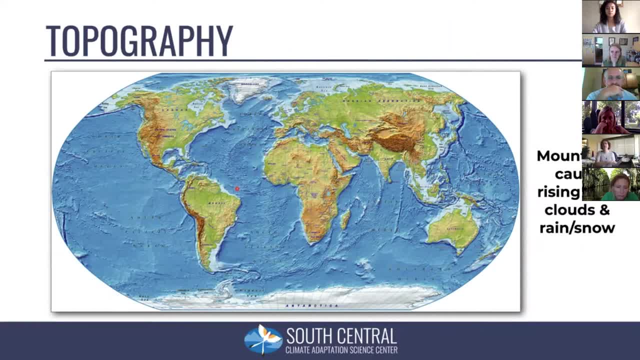 you're gonna hit clouds and the possibility of rain, And so if you, for example, here are in the United States and we have generally westerly winds and so every system that's coming off of the North Pacific Ocean that's gonna be shoved up, these rocky mountains. 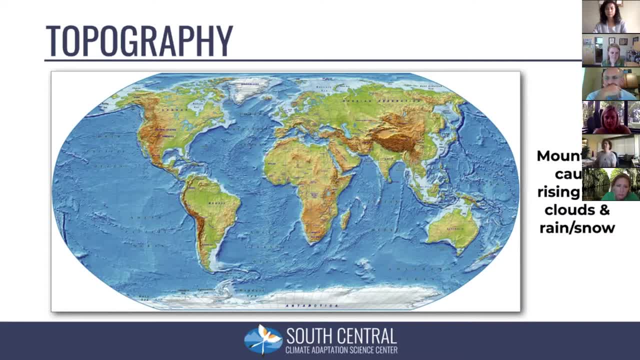 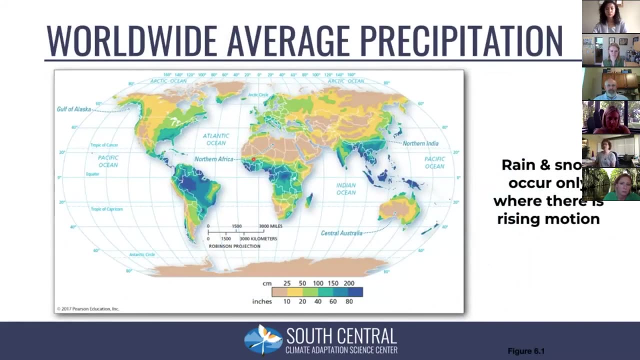 and when it's shoved up it's gonna rain, And then on the other side that air is moving downward, and so generally we get clear skies when we have that, And so that's where we see a lot of our patterns in our precipitation. 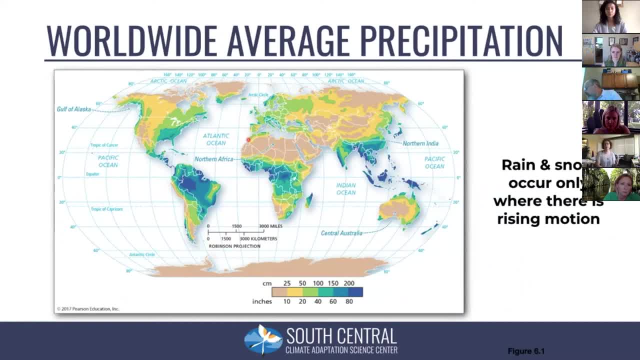 So these precipitation patterns, just like everything else in the climate, is just a result of physics. So part of the physics is having rising motion at the equator, at that intertropical convergence zone. Part of those equations of physics show us that rising motion here in the very far western. 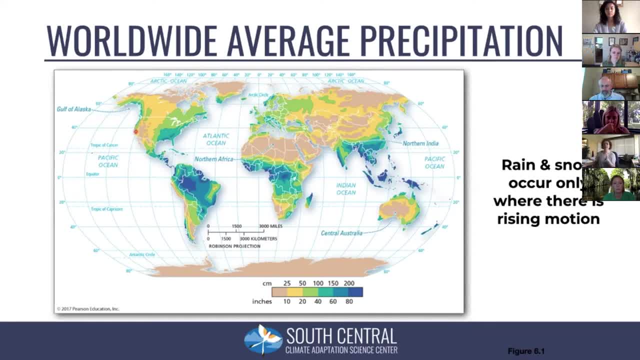 part of North America is going to give us precipitation. Then we're going to have drier air in the Great Plains and then, as we get a circulation that moves maritime moisture to the east coast, we get another area here of precipitation. So all of that is just a result of the physics of the system. 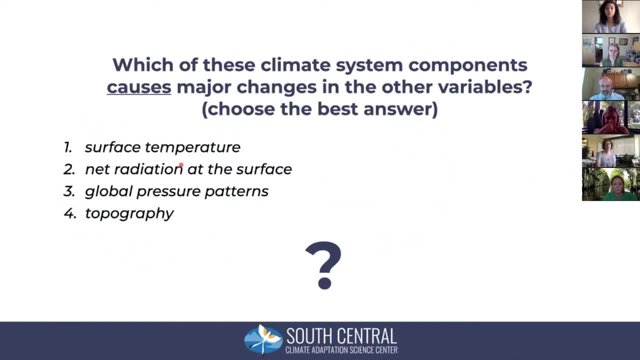 So here's your next question. So, of these components, which is the one that's kind of the driver that's causing changes in the other ones? Okay, great, Okay. so I think we have most people who have given their answers. 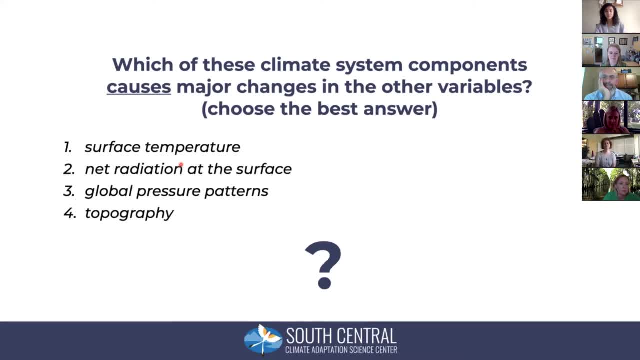 So if we'll end the poll and show the results, then what we see is: most people said it's the net radiation at the surface and that's correct. So that balance of incoming and outgoing radiation is the net radiation at the surface and that's. 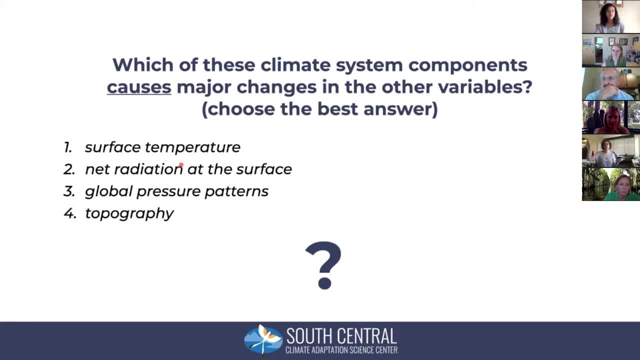 correct. So the net radiation that's coming and outgoing energy, depending on what latitude that you're at- is going to be driving all of the other things, including the surface temperature. So surface temperature is really important, but it's also driven by that net radiation. 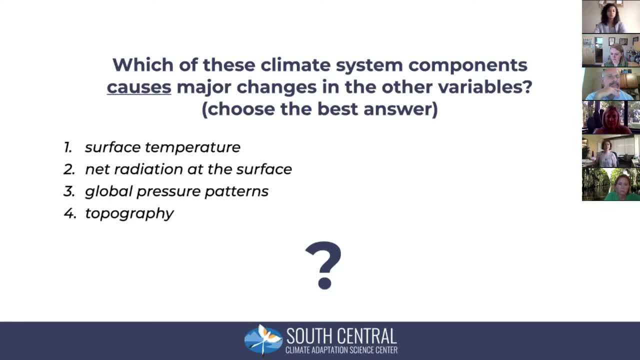 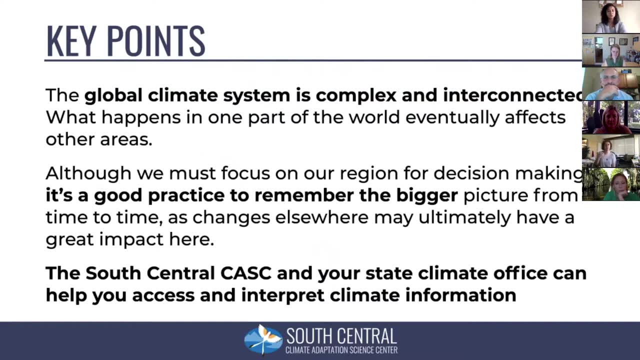 that occurs at the surface. Okay, So the key points for this area is that our system is pretty complex and interconnected, So one of the things that's very hard for climate scientists like myself is messaging about climate change, because it's so complicated. It's not like a. you know, I tripped over a curb and I fell on my face. 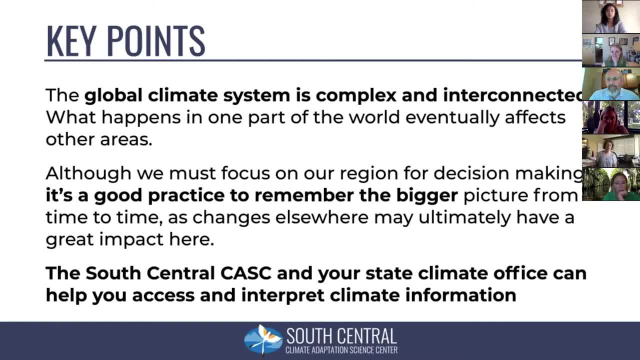 That's pretty easy to describe. So this is a complicated system And it's helpful to think about the big picture, Okay, So I encourage you to think about the big picture, even when you're zooming in to your local decisions. So don't get so localized that you aren't thinking about how this is being driven by. 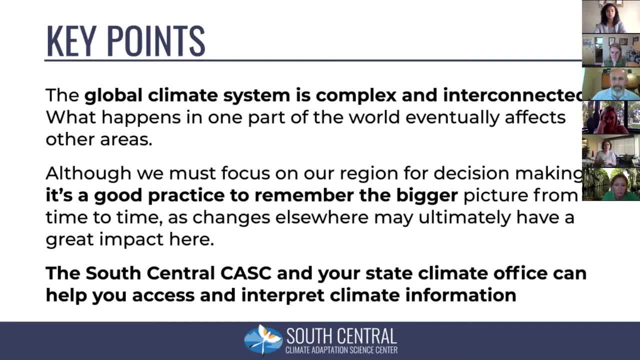 the big picture. So I encourage people to keep looking at some of those broader global climate model projections, even at the time that they might be diving deeply into the regional climate projections at a point- And you don't have to do this yourself, Okay- 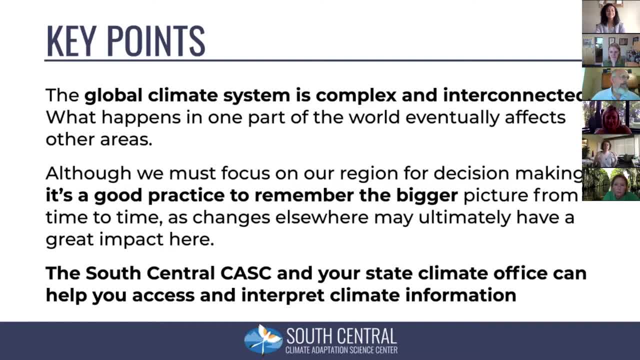 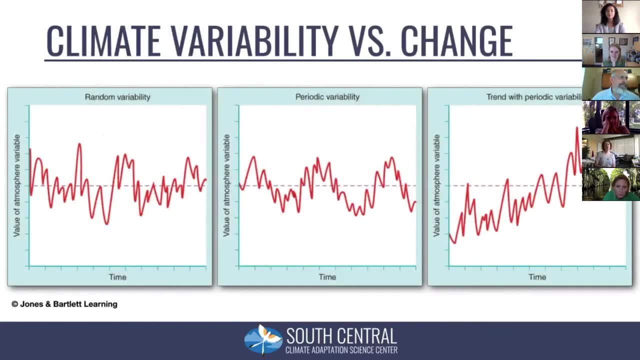 There are people like Monica and Derek and Adrian and others who are here to help, And so please just get ahold of us and that's our job: to help you out. Okay, So another clarification on terminology. we refer to climate variability versus climate. 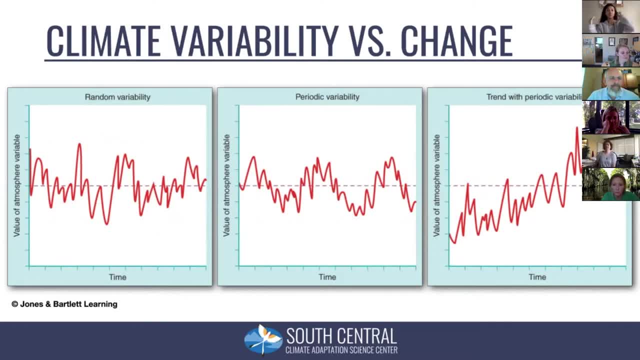 change, Climate variability, is happening all the time. So, especially if you live in the South Central part of the country, you're very used to different kinds of weather systems moving in and changes that could be. you know, from one day to the next you could have a 40 degree Fahrenheit change in temperature and you go from clear. 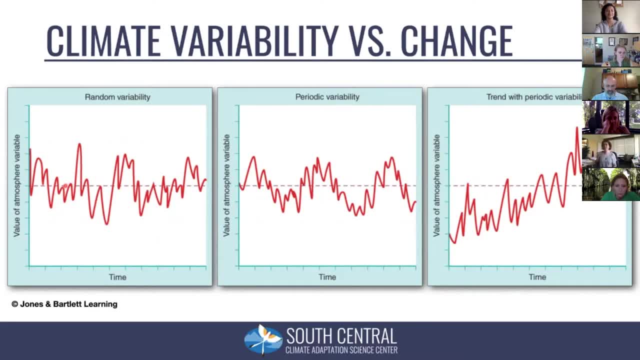 skies to a deluge of pouring rain. That's our climate variability, That's the system, that's internal to the system And in some places that's a fairly random occurrence. but in most places we have the random day-to-day variability superimposed on to some sort of cycles. 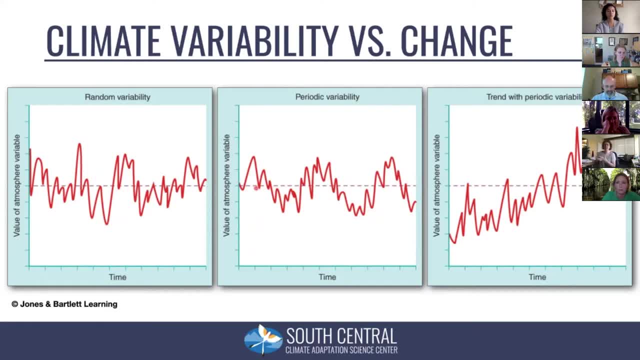 And so this cycle, for example, if you think of this variable as temperature, this cycle could be El Niño versus La Niña. So we see global temperatures increase. We see global temperatures rise. We see global temperatures decrease during El Niño years, decrease during La Niña years. 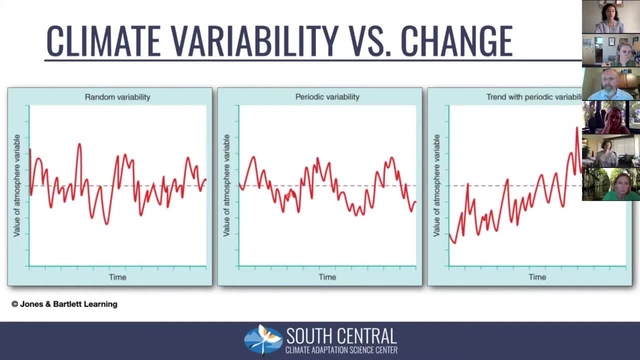 And we get the El Niño-La Niña cycle every three to seven years, And so there's some sort of cycles that are occurring there. Climate change is a trend, So we'll be focusing on that trend today, but remember that trend still has the cycles. 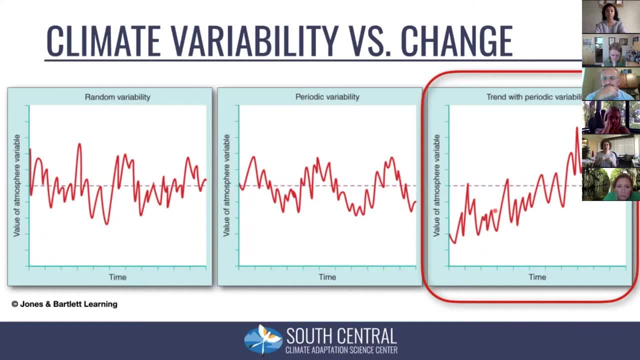 and it's still a trend. It still has the random variability involved in it. So the random variability could result in this next winter being the coldest winter we've ever seen, wherever you are. That's just part of the variability. this change we look at on a decadal to century. 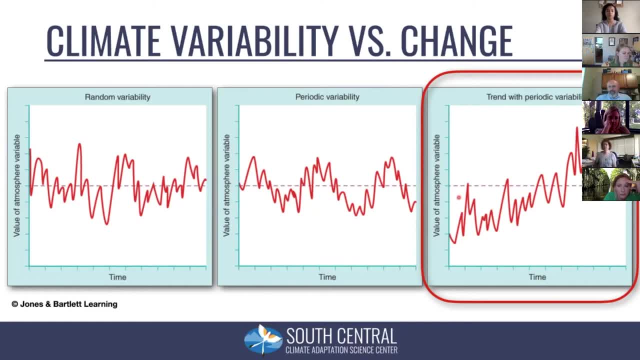 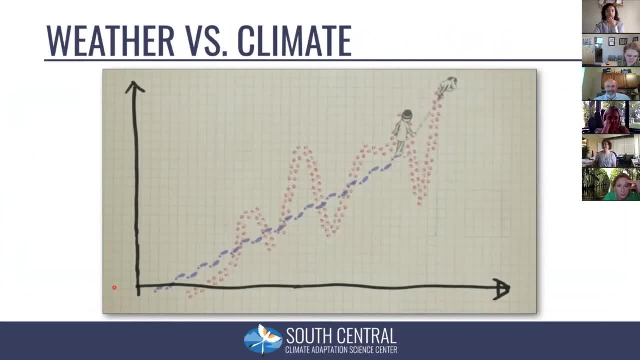 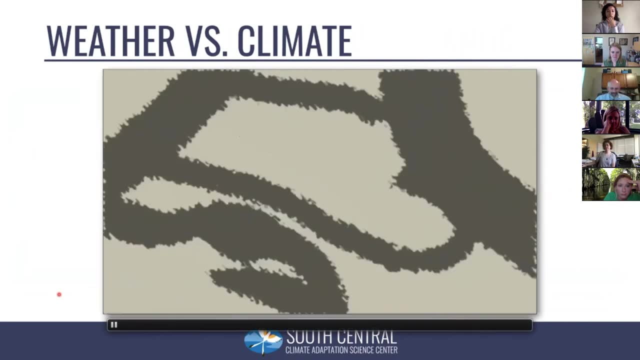 or longer time scale. So have a little movie. Hopefully you will hear it. I think I clicked the right buttons. A common mistake when interpreting statistics is to look at them from too short a distance. This can make everything unclear and confusing. So forget the details and take a step back. 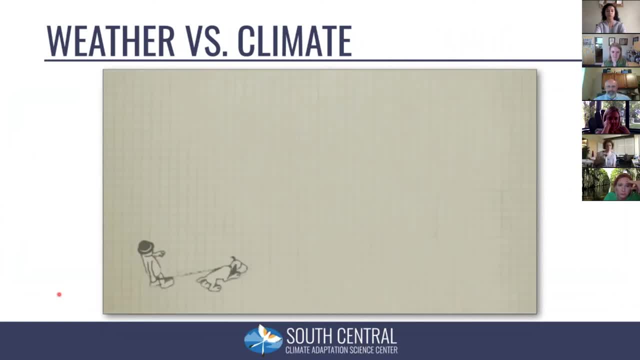 You're looking at the dog when you should be concentrating on the owner. As you can see, the dog is all over the place, leaping and bouncing, sometimes upwards, sometimes downwards. But where do you think it will be in 10 seconds time? 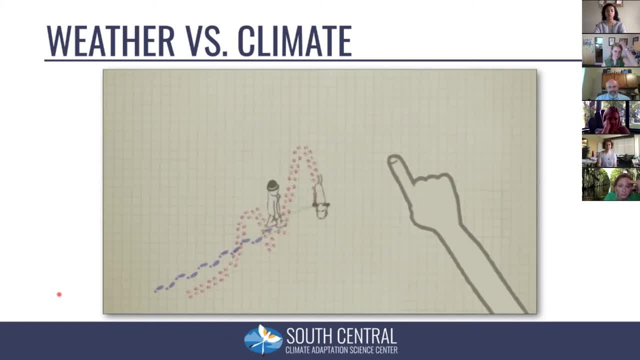 Around here, right, But at this moment the dog is on its way downwards, so why do you think it will find itself up there? It's because you've noticed the owner. The owner is the trend and it's he who determines where they both will be in a while as a bit. 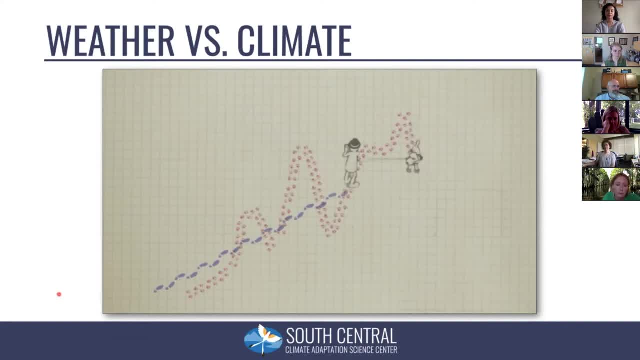 longer than a couple of dog bounds, He could change direction. there's a lot we don't know about this guy, but everything we do know indicates he's heading in that direction. The owner is the long-term trend, the dog is the variation around this trend, or the 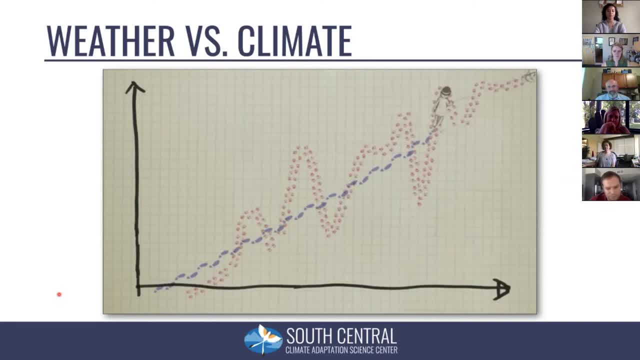 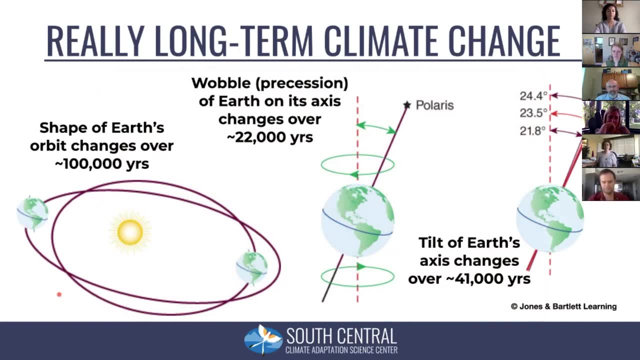 owner is the climate, The dog is the weather. All right, so both of those are going to be important to all of you, but just good to keep that in mind. Also, today and tomorrow, we're going to be focused on climate change as it results from. 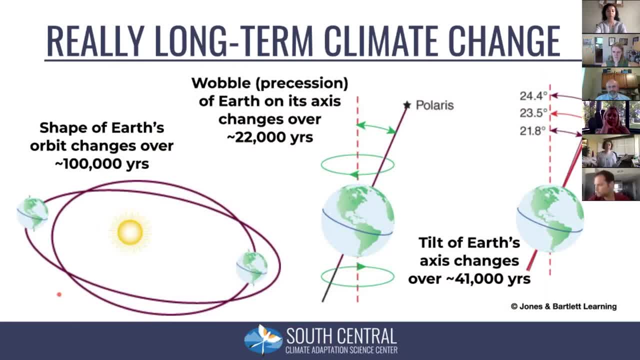 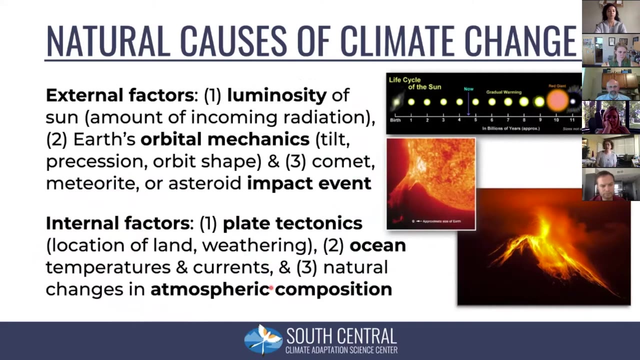 human causes. There is also climate change. that's natural. For example, change in climate Change in climate, Change in climate, And we did see that change in our orbital mechanics result in the major glacial periods that we've seen over hundreds of thousands of years. if we get hit by a comet, which 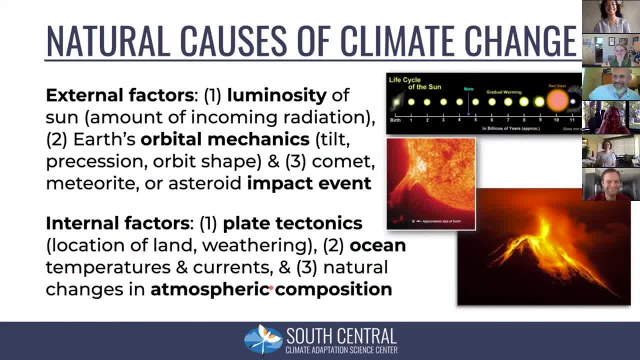 I shouldn't talk about, because 2020 has already been a year of every disaster possible. But I'm going to say Bruce Willis will go save us if we get hit by a comet this year. So there are things that are natural causes and we see that in our climatic history. those of you who said you mentioned you. 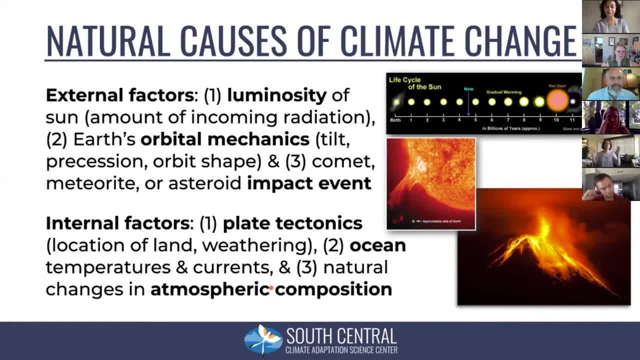 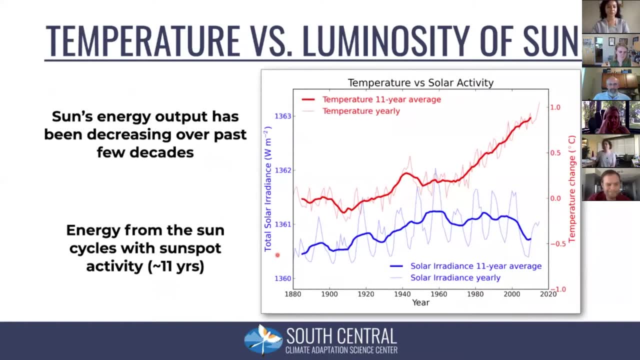 Geologists, you know this, But this is really really long term. We won't be talking about that in this section. and Some people talk about: well, the sun's getting brighter, or we're in this, We're in some sunspot cycle or what, what have you? So we also won't be talking about 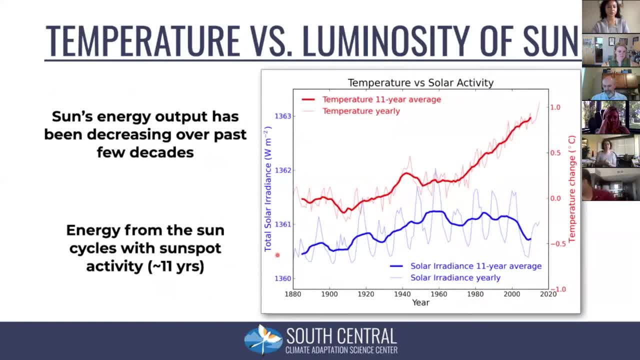 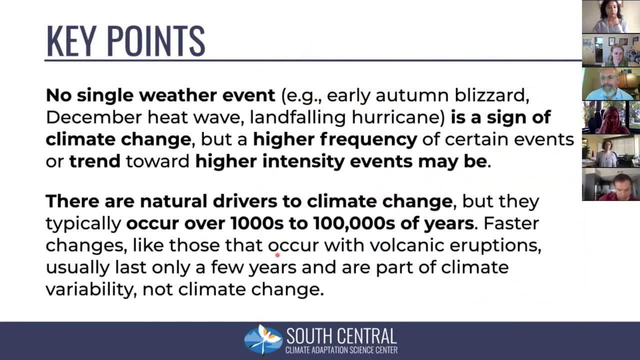 Changes in luminosity of the Sun. In the past few decades. this is actually decreased, not increased, but during that time we've seen our global average temperatures increase. So Just a reminder: no single weather event is going to be, You know, Caused by climate change, but every single weather event has a climate change signal in it. today, 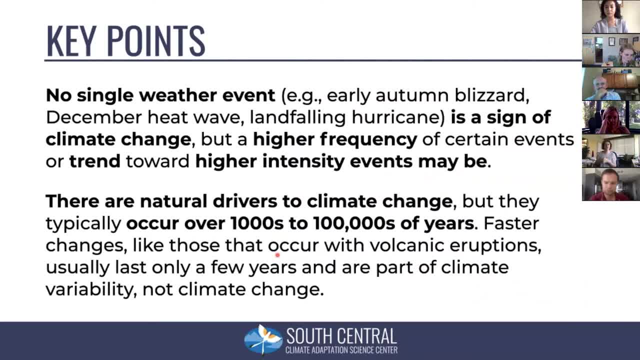 And So we, as climatologists, are looking at Long-term trends, we're looking at changes in the frequency of different types of events and, specifically for many of you, We're looking at intense events, things that cause severe changes in Ecosystems, for example, And yes, there are natural drivers. 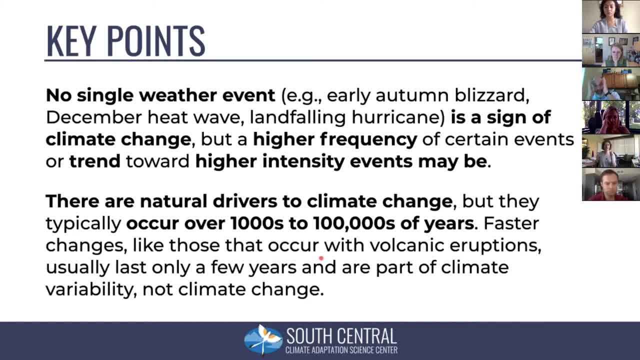 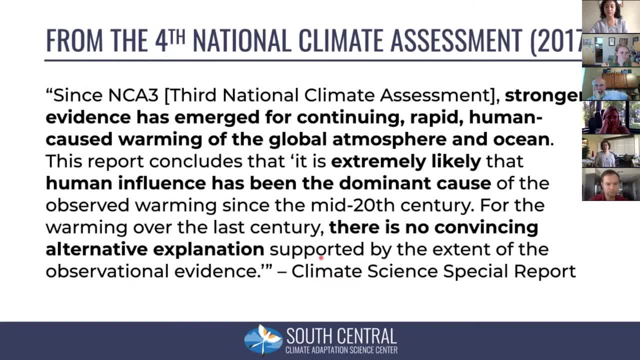 But our changes are occurring faster than that and we can determine where they're coming from, and so focusing on Anthropogenic or human-caused climate change is much of what we see and what's called the national climate assessment. this has The most recent version, has shown stronger evidence. 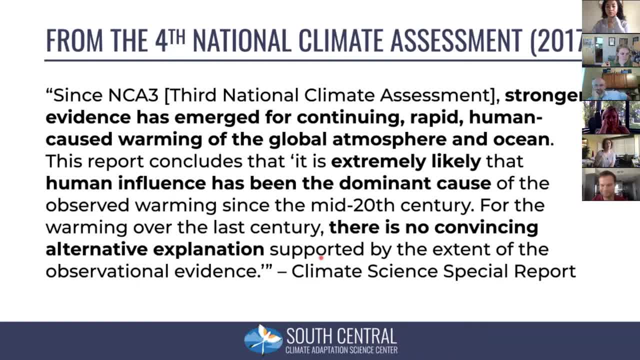 For continued rapid human cause- warming of the global atmosphere and ocean- Extremely likely that human influence is the dominant cause, And then there's no convincing alternative explanation. So, believe me, there are enough climate scientists out there that anybody who comes up with a possible cause That's different from what we're going to be presenting today. 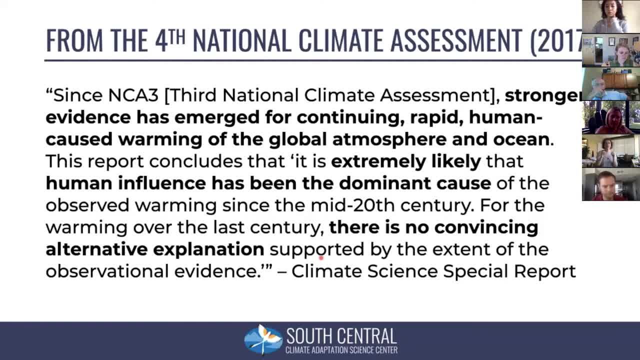 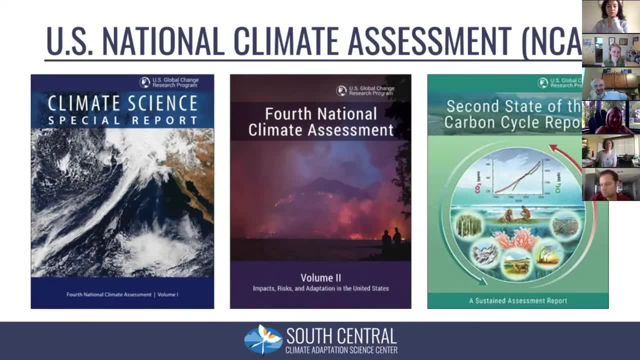 What we're going to be presenting here. that has been, that has been tested and proven Incorrect, So there is no convincing alternative explanation. Don't count on Facebook to be your source of climate and weather information. Certainly look at the wealth of reports through the national climate assessment. 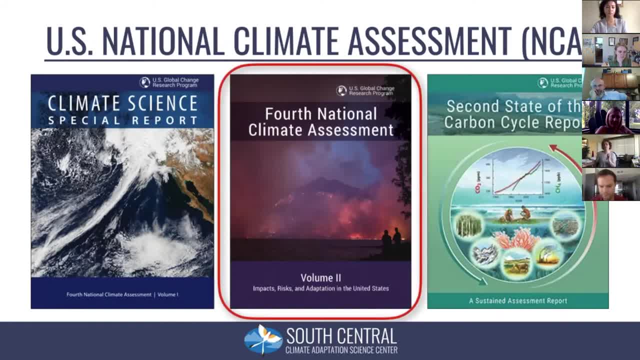 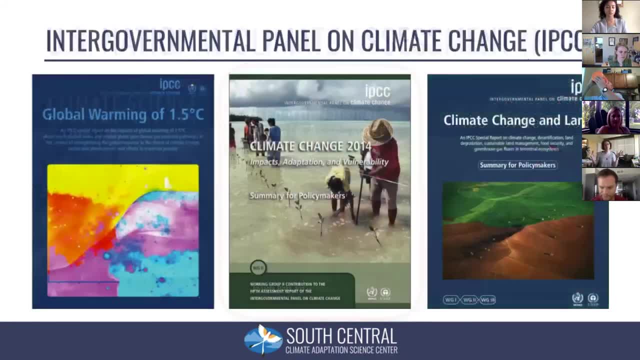 including, most importantly for all of you, this report on impacts, risks and adaptation. and if you're interested more broadly in the world, we have Access to the Intergovernmental panel on climate change reports And again, it has a report that focuses on impacts and 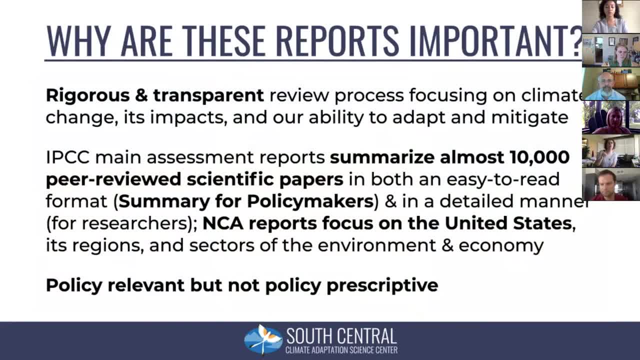 adaptation. And the reason why these reports are so important is because they're rigorously Reviewed, they're transparent, They're open for public comment. Every public comment has to be answered by somebody on the science team and that answer has to be publicly available for anybody to challenge. 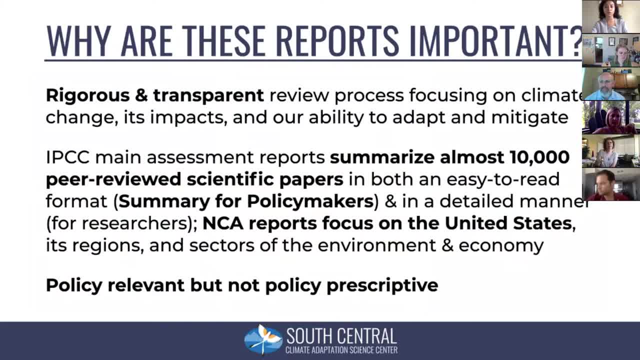 Those reports are not doing their own science. They're summarizing the science that has gone through the scientific peer review process over the decades. It's basically, you know, trying to ensure that the time that you take is focused on the things that you need to do and not going to 10,000 scientific papers to try to figure out what's going on in our climate system. 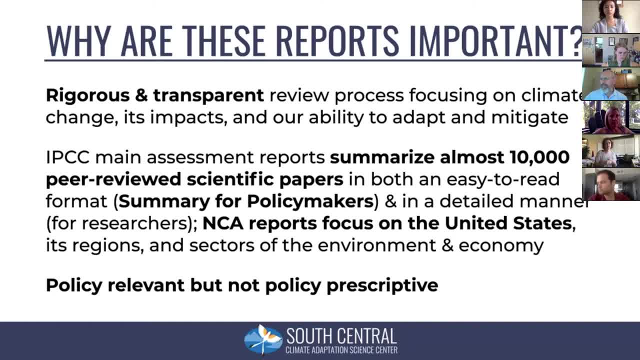 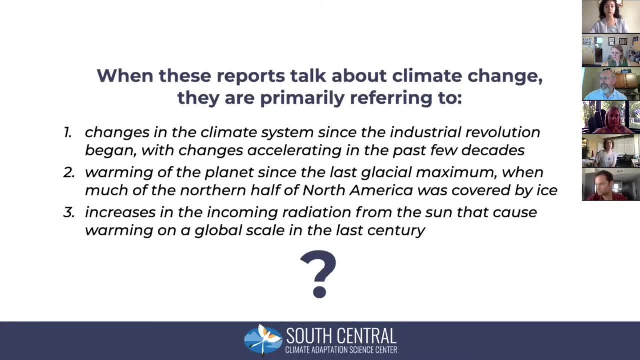 So I highly recommend These reports. they're meant to be policy relevant, but not policy prescriptive. We don't tell you what to do. We summarize the science For you. So when these reports talk about climate change, then what do you think that they're talking about? 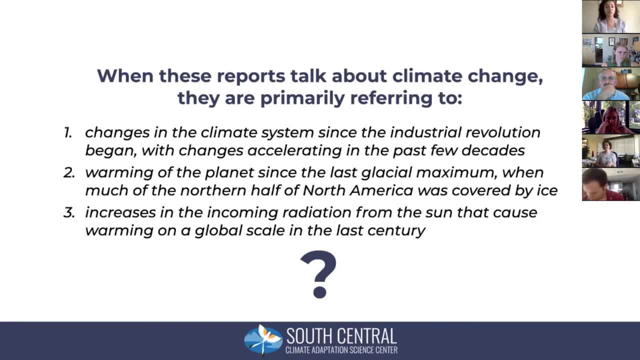 When these reports talk about climate change, then what do you think that they're talking about? All right, so we will close that poll. And, yes, most of you got it. They're talking about the changes in the climate system. So these are all the different components. 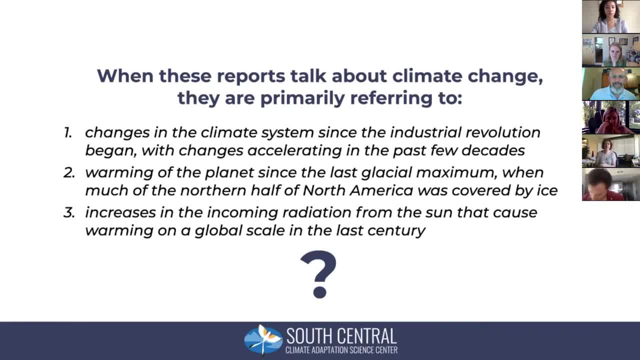 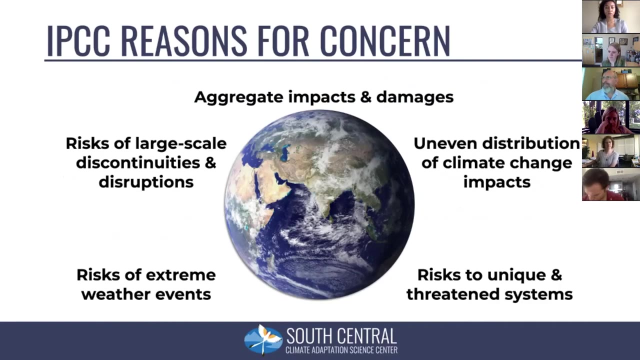 of the system and the changes that have occurred since the beginning of the Industrial Revolution. They do focus on the last several decades because that's where we've seen a lot of this acceleration of these changes that occur, And the reason why these are important is itemized in this Intergovernmental 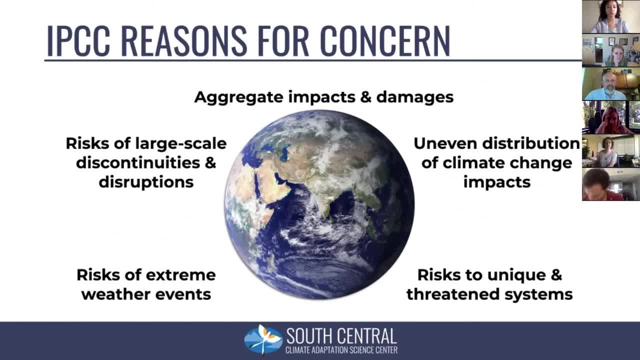 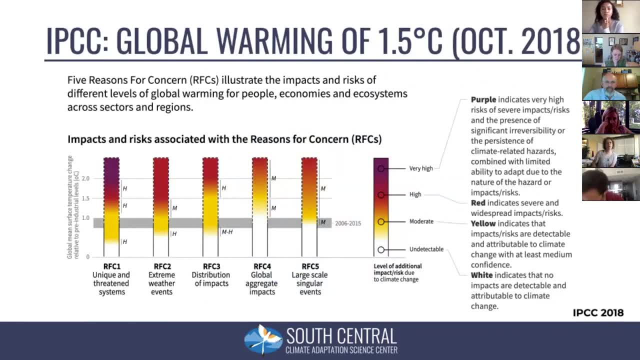 Panel on Climate Change report. There's five areas. I'm not going to go through them in detail just because of time here, but I do want to highlight a recent report called Global Warming of 1.5 degrees Celsius. This compares what will. 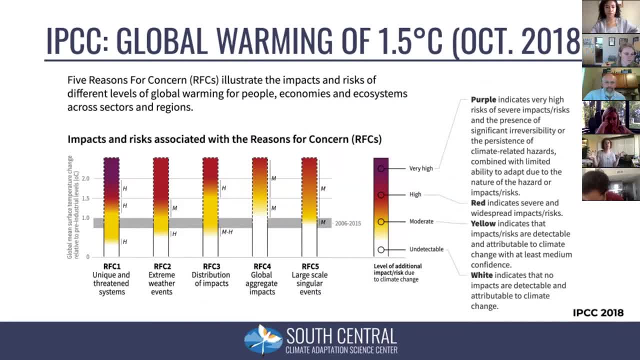 a warming of 1.5 degrees Celsius on average across the globe look like in comparison to the Paris target amount of 2 degrees Celsius? And I'm going to give you a little bit of an overview of what that looks like. And I'm going to give you a little bit of an overview of what that looks like. 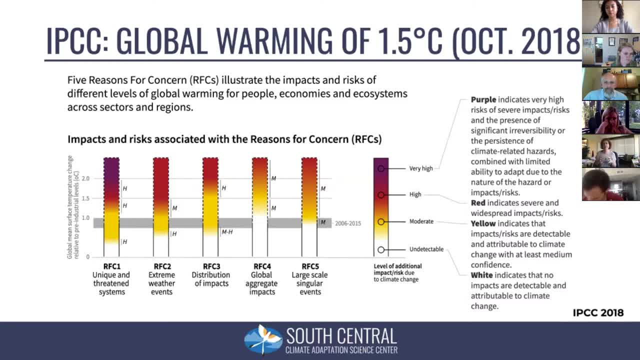 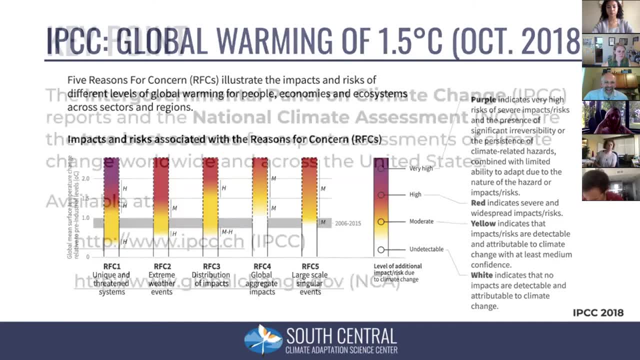 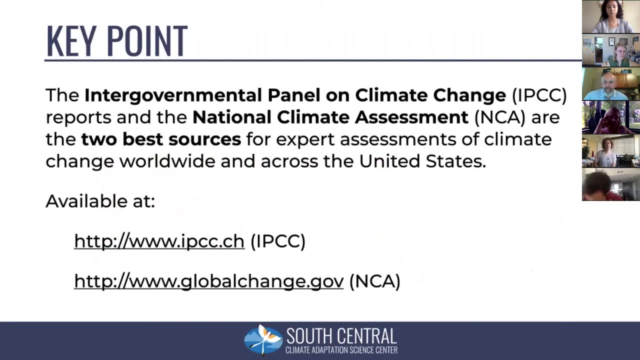 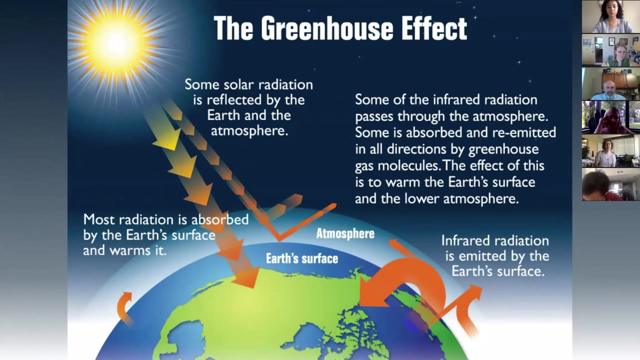 And it'll show you where the threats are changing and how high or low of a risk in some of those major areas, And so these are the reports. This will be included in the material that you can access, And those are all available online. All right, So real quickly. this is the crux of our human-caused. 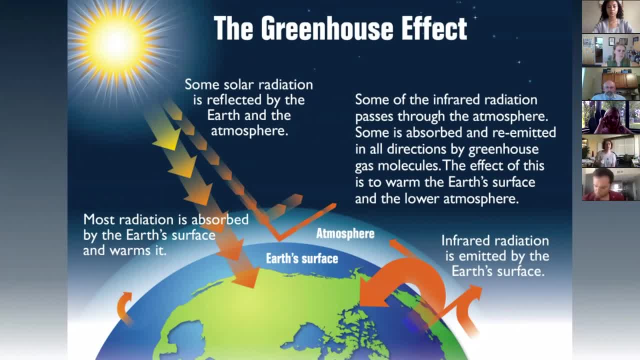 change in our climate system. Okay, The greenhouse effect. as I mentioned before, our solar radiation is primarily in the visible and ultraviolet wavelengths. The atmosphere is mostly transparent to that. So that means that most of that solar radiation makes it to the surface. There's some reflection that gets rid of. 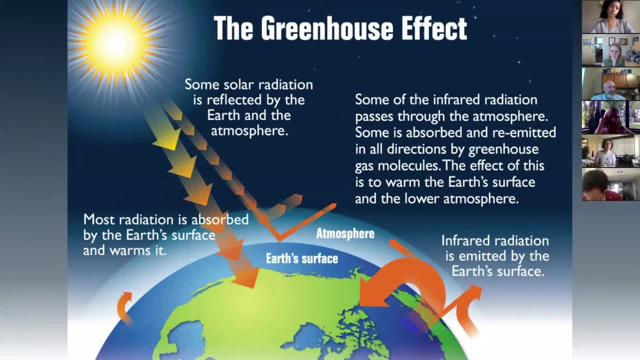 some of it, but it mostly just moves through our atmosphere, The infrared radiation that results from emission from our Earth. so our Earth emits in the infrared. that radiation is highly absorbed by these greenhouse gases that I named before. So that means that as that radiation tries to leave our planet, our atmospheric system, 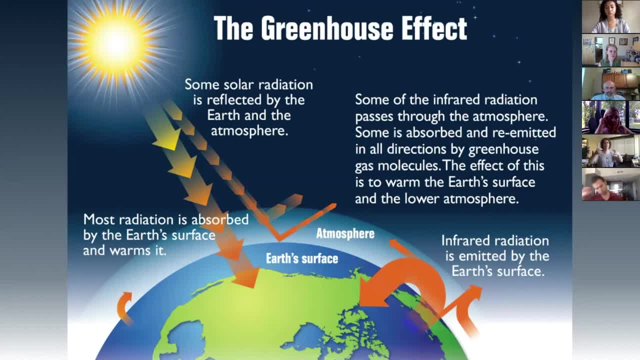 it's absorbed heavily in the atmosphere, naturally by the natural occurring greenhouse gases, And then those greenhouse gases re-emit that energy, half of it upward, half of it downward. The half that comes downward warms our surface. Okay, And without the greenhouse effect. 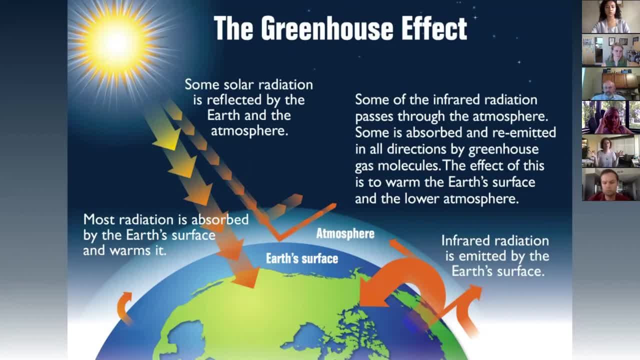 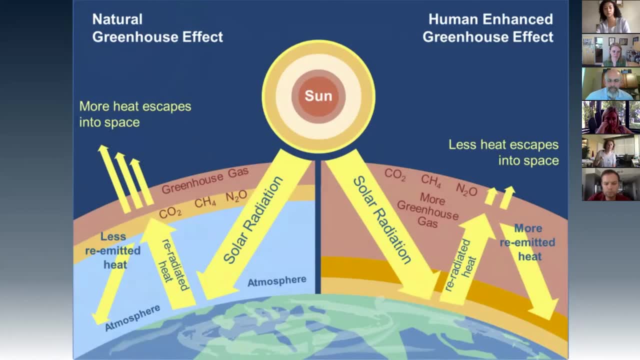 Okay. So the thing that we add more greenhouse gases than has been natural. So the left side of this diagram is our natural greenhouse effect. The right hand side is when we add more greenhouse gases and then there's more absorption, There's more re-emission to the surface and that's more energy going into the surface. 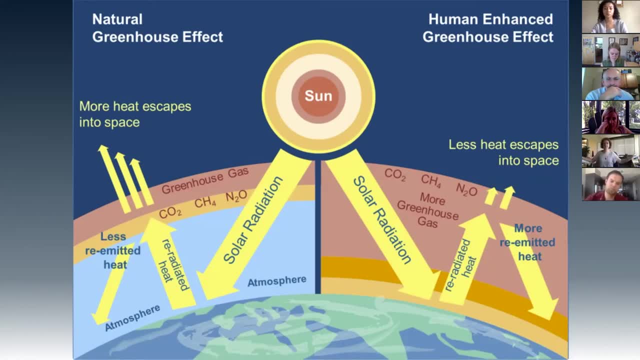 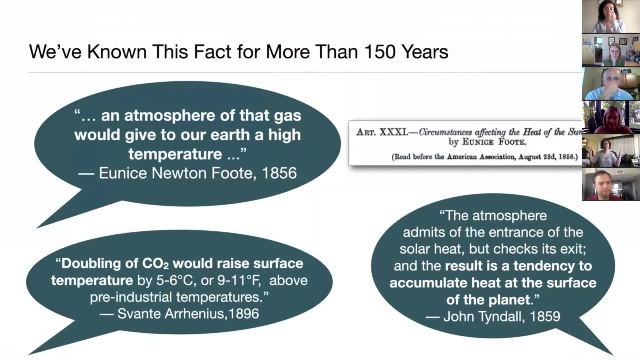 raising our temperatures more and then our temperatures act on the rest of our climate system more And with that, redistribution of energy and all of the things we talked about earlier- And this is not a new concept. This does not start with any political party in the United States or anywhere else in the 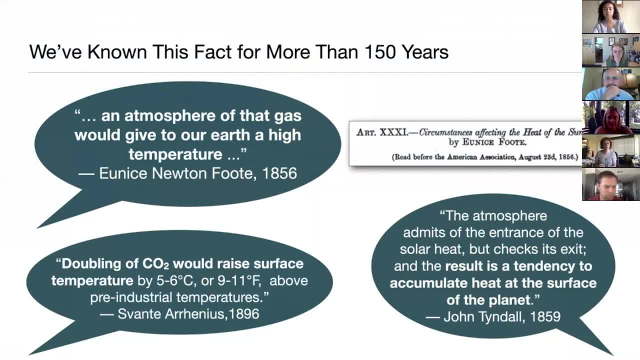 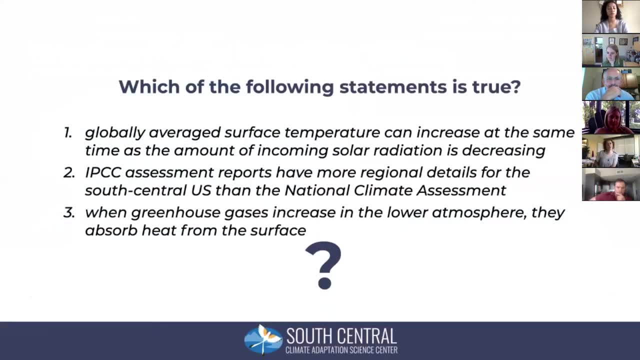 world. This started from science over 150 years ago, So it's been known for a long period of time. So our next question is: which of the following statements is true? Which of the following statements is true? Okay, we'll go ahead and end this poll now. 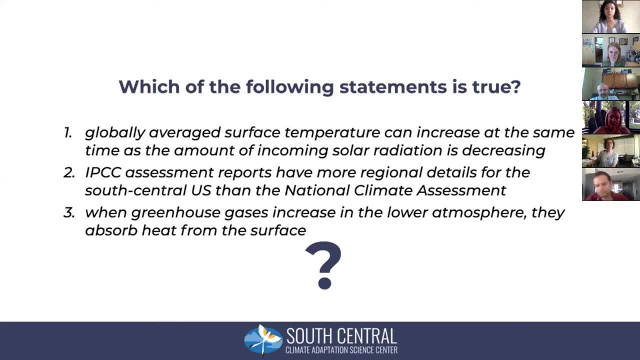 I see that I probably didn't word this question very well, So we got equal numbers on this. So it is true That the global average temperature can increase at the same time that we see the amount of solar radiation decreasing. That's actually what's happening now. 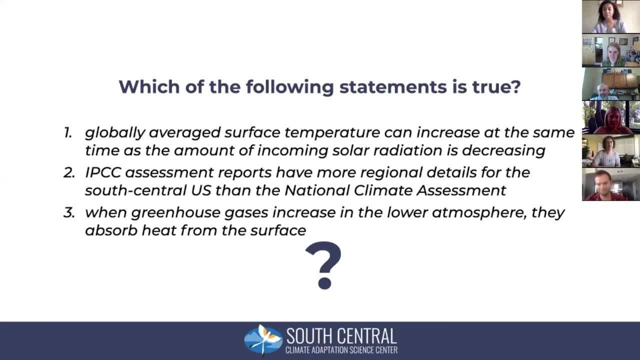 We're seeing less incoming solar radiation, but our temperatures are increasing. The greenhouse gases are absorbing the heat. I meant I should have said at the surface, so that that would be a wrong answer. They're absorbing the heat that does leave the surface, but they're absorbing that heat. 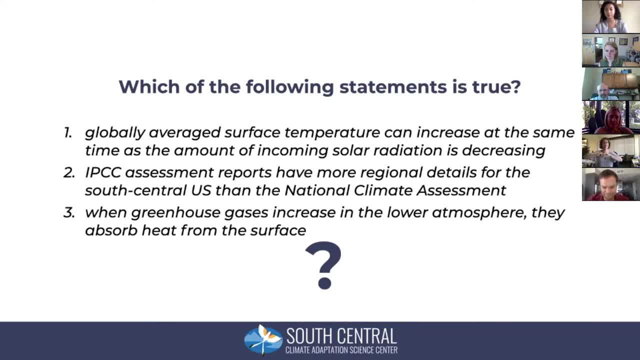 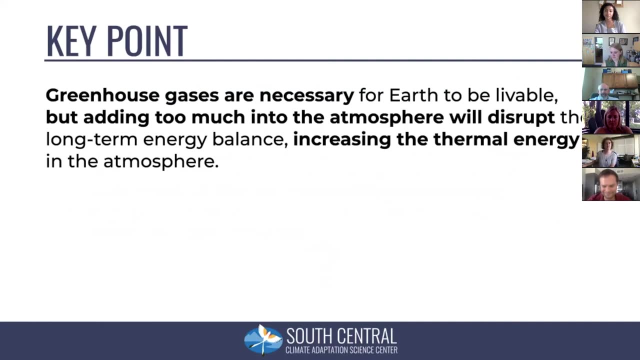 in the atmosphere, in the lower atmosphere itself, And then they're re-releasing that heat. So Renee mark herself negative points for poorly worded question. So those greenhouse gases are necessary, but we're adding too much to the atmosphere. 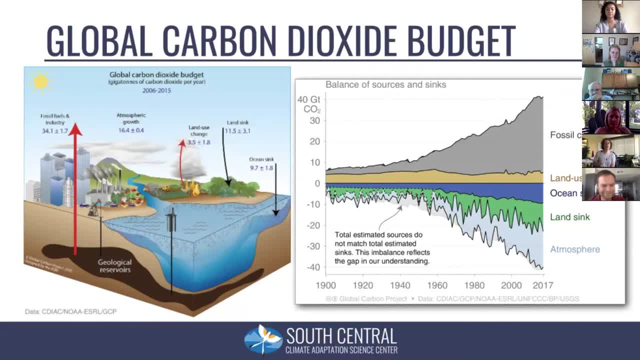 And where are we adding that from? So we're going to focus on carbon dioxide here. So we know we still have greenhouse gases that are increasing for methane and nitrous oxide and others- But if you look at the percentage of gases that are causing this, carbon dioxide is the 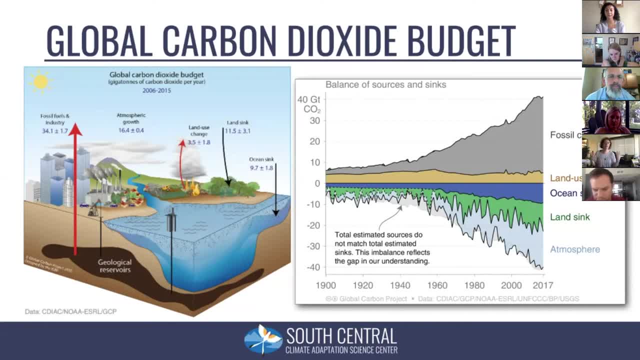 main one. And so where do we get carbon dioxide? Well, we have carbon dioxide in our natural systems, and there has always been, in our past history, a natural balance between the carbon dioxide coming into the earth's surface and that that's leaving the earth's surface. 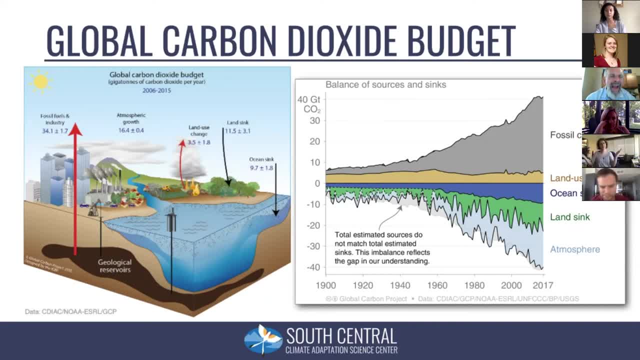 So, for example, forest fires will release carbon dioxide, that's natural. The oceans absorb carbon dioxide, that's natural. But over a long, long period of time this got to be a nice balance at the surface of incoming and outgoing. What changed? 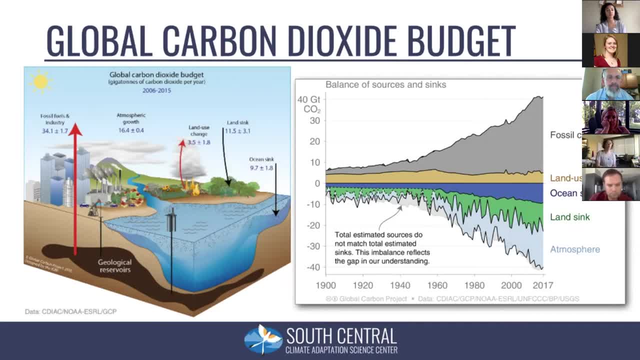 What changed? Because humans started going below the surface, taking geological reserves of carbon, either in the form of coal or oil or natural gas, bringing it to the surface. If that's all we had done, not a problem, but then we burned it. 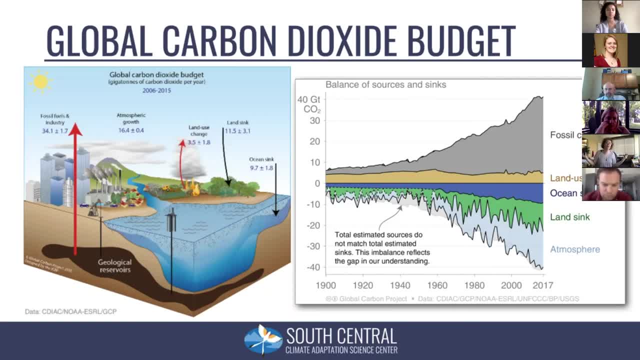 And we burned it for good reasons: for energy. our economy results from that burning, So we're living in much better conditions than we would have had we not done that. So that's great, Except for it does have a long-term impact. 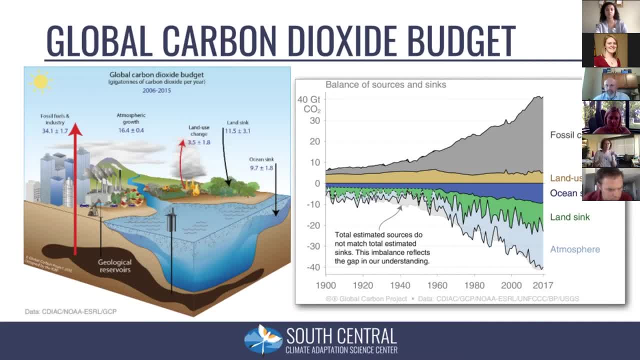 And that's because, unlike water vapor, which all of you who are working in water know that our water cycle kind of works the water out of our atmosphere. in a matter of a couple of weeks, carbon dioxide and some of these other greenhouse gases sit in the atmosphere. 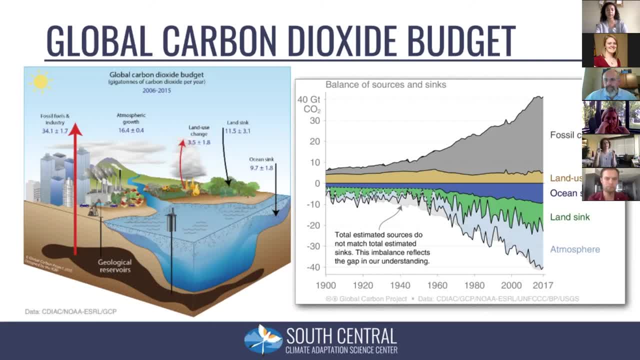 for a long period of time, On the order of tens to hundreds of years. So that's great, Except for it does have a long-term impact, But unlike water vapor, which all of you who are working in water cycle in a matterв. 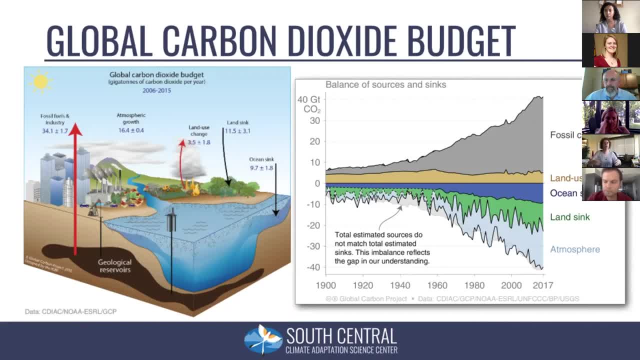 of years. carbon dioxide and some of these other greenhouse gases sit in the atmosphere for a long period of time. So that's great, Except for it does have a long-term impact. So that's great, Except for it does have. apart from that, for speaks nächste slide, carbon dioxide—. 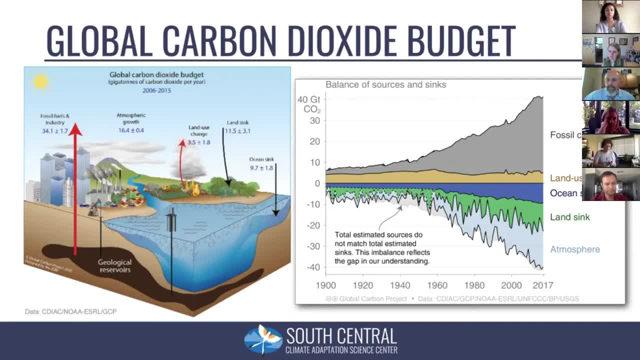 carbon dioxide's interaction with other em. ampere goes from zero to a hex- teaches Na entering ion— and our earth system is trying its best to remove that. so again, the ocean tries to remove carbon dioxide. our vegetation, so what's labeled here is the land sink. 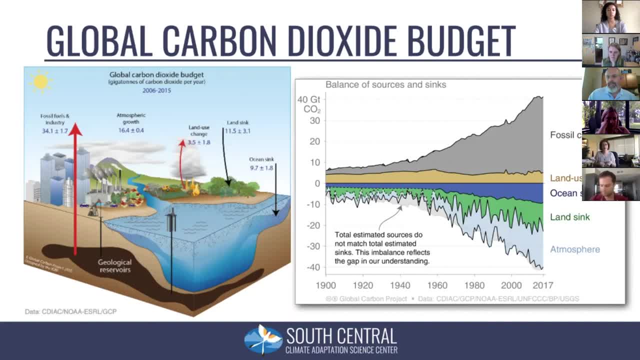 the vegetation is trying to remove carbon dioxide from the atmosphere, and it just can't keep up. so the ocean and land together are removing about half of that excess carbon dioxide, but the rest of it now is accumulating in the atmosphere, and that accumulation is getting greater and greater for each. 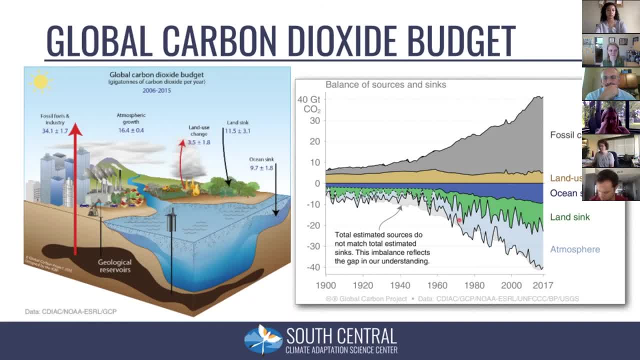 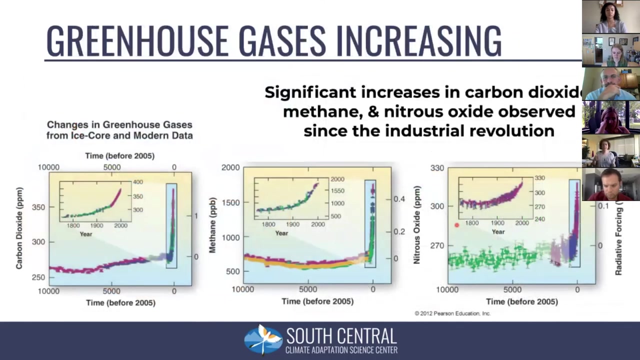 decade that we go through, and even if we shut it off today, that excess carbon dioxide is going to be in the system. so that's why our Center focuses on adaptation. so we know that we are going to have to live with climate change for the rest of our careers, and so we see in the long-term. 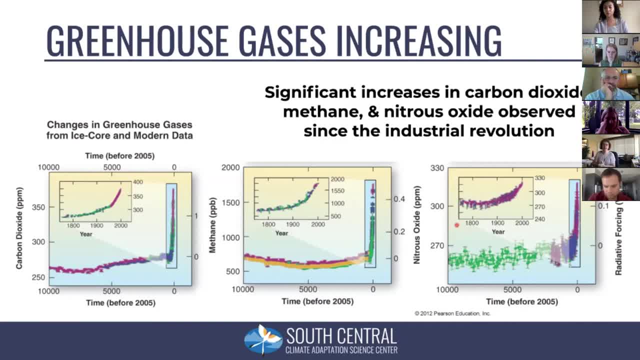 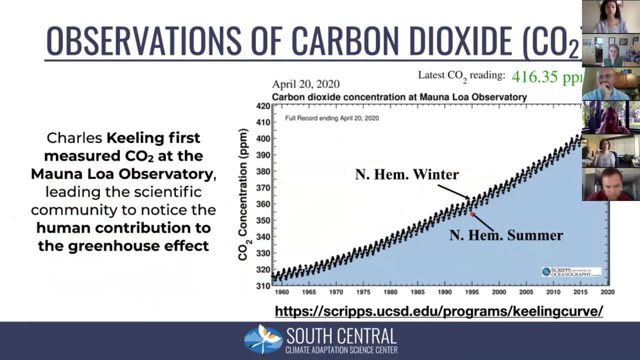 record that skyrocketing increase of carbon dioxide, methane and nitrous oxide. all of these are long-lived gases. methane has a shorter lifetime in the atmosphere than than the other two, but but we're seeing in all of our measurements, on average, globally, we're seeing this increase in the carbon dioxide. so this 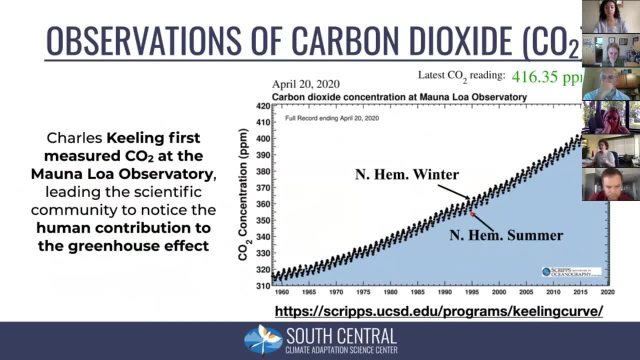 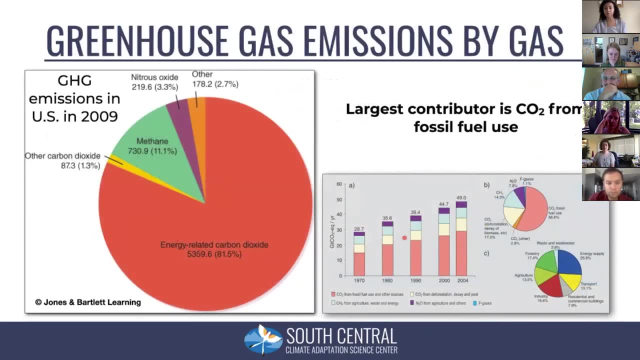 is the fingerprint of the burning of the fossil fuels. we still see our natural cycles as our earth system kind of breathes in and our carbon dioxide over the seasons. but most of the greenhouse gas emissions that are occurring, that are still staying in our atmosphere for a long period of time, is 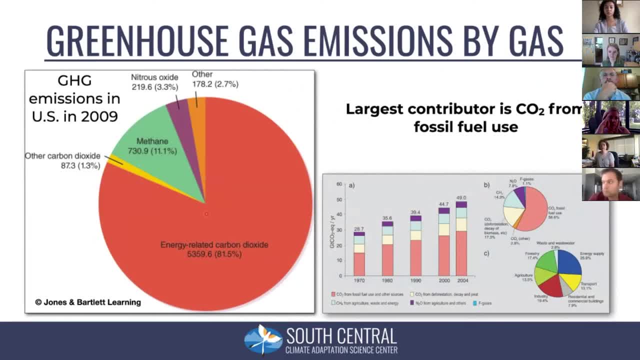 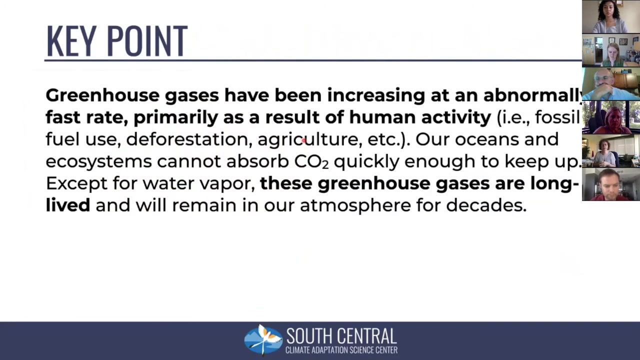 energy related carbon dioxide. again, methane is a still a major part of it. so this is primarily through also fossil fuel use, but also through intense life, livestock agriculture and what we're seeing through multiple methods that I didn't go into here. we are seeing that human fingerprint on our atmosphere composition and again, as 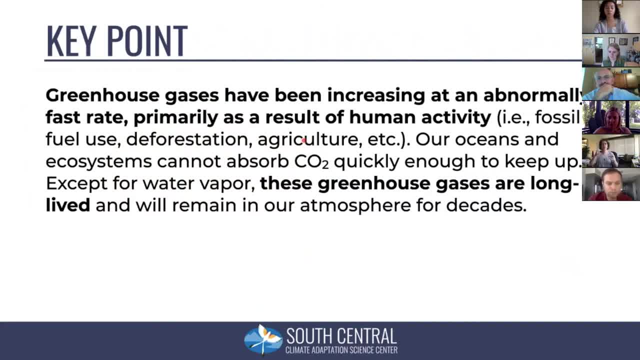 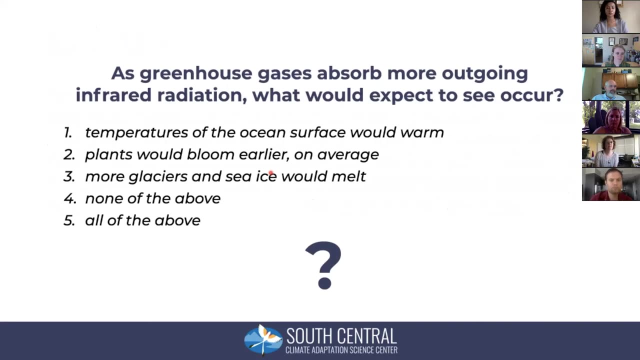 I mentioned at the very beginning, anything that happens to change that energy budget in our system is going to change everything: the temperature, the precipitation, the wind patterns, all of that because they're interconnected, all right. so hopefully that means that this question will be pretty straightforward for all of you. 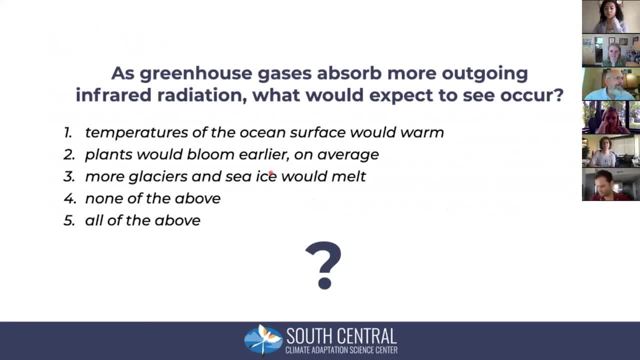 okay, so we'll end that poll and show you the results. so, yes, the because of the interconnection of that earth system, that changing one component of it and the most important component, that net radiation that we have in our system, changing that will change all over the world, and that's what we're going to be talking about in the next couple of minutes. 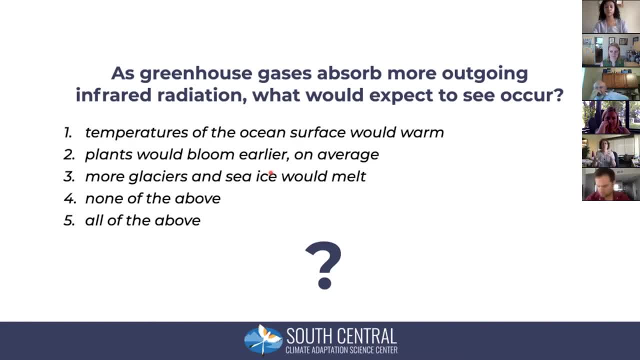 okay, so we'll end that poll and show you the results. so, yes, the because of the interconnection of our climate system, and then our climate system will have caused changes in other natural systems that we have here on our planet. so we refer to those as indicators. so so the question is okay. 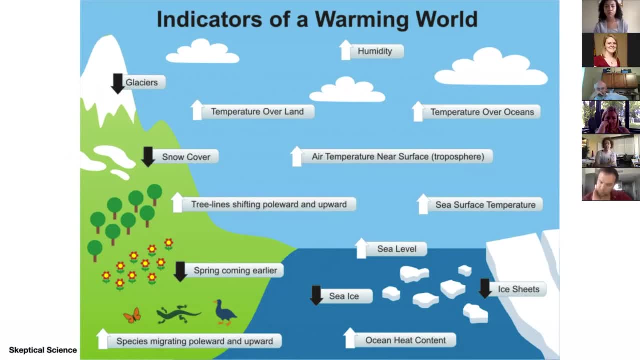 so our science tells us that these greenhouse gases are increasing. we're measuring that, and the science tells us that an increase in greenhouse gases will cause more energy to be absorbed in our earth system. and if more energy is absorbed in our earth system, then that means our earth system should warm. and so what should we be able to measure if we have a warming world? 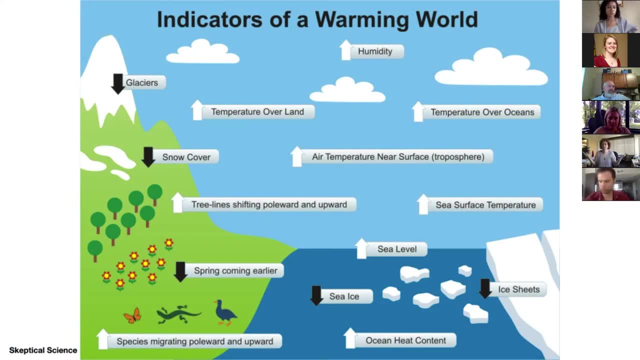 so if we have a warming world, obviously we should measure increases in temperature, because it's warming um, but not just temperature in our air by the surface, but we should also, since that atmosphere is touching the top of the ocean, the sea surface temperature should be increasing and the increase. 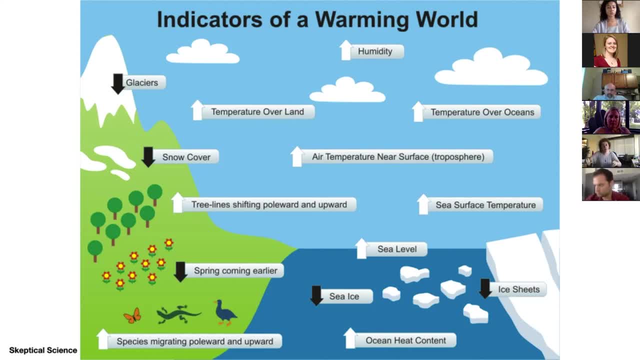 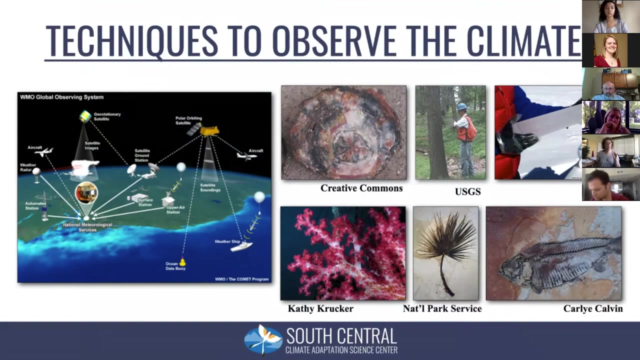 in ocean temperature should be greater at the surface than below. so we know that that energy is not coming from some deep volcanic activity. um, it's coming from the warming of our atmosphere, and this whole host of other things should be happening, so are they? so we measure them through. 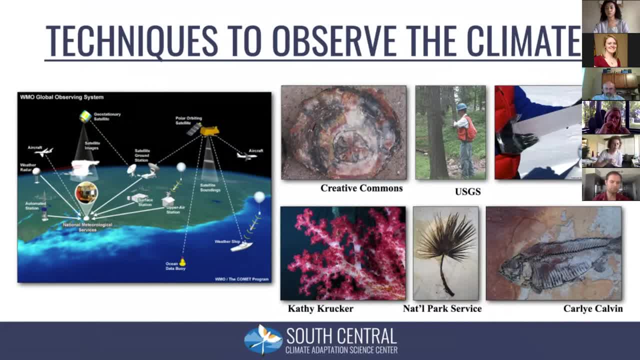 various techniques. we have all of our, you know, very sophisticated satellite and radar and um, even to the back backyard rain gauge, all of that data coming in, um. but we also have signals in our geologic system that are coming in, and we also have signals in our geologic system that are coming in and 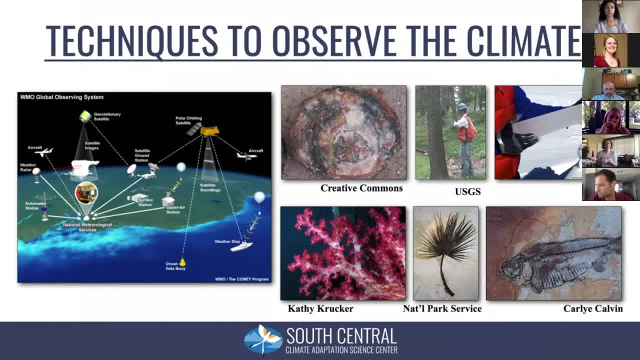 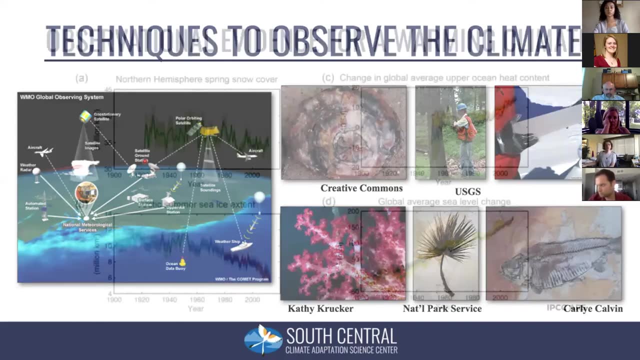 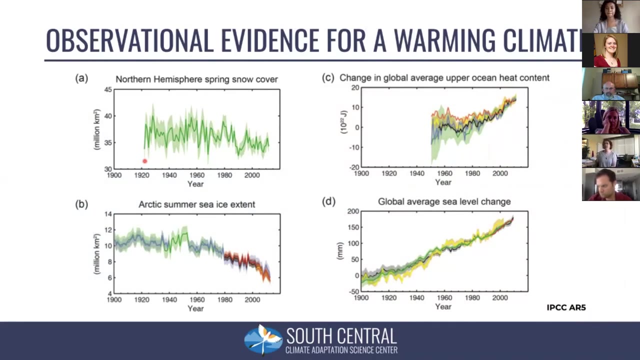 um, not cold, butínhassis, that i call a long range system, really. um, so we can see the temperature thing, like you know, after 20 inches, and you can see that again by counting the layers as you go back. historical um, history, um, and, for example, in our ice cores, where. little bubbles of the atmosphere were trapped um years and years ago so we can see what our atmosphere was like um, and so we use all of that to see: are these things changing? that we expect to see changing, absorbing. we think that over all the snow cover, across all of our爱ves, bedland, we see we can pull those. 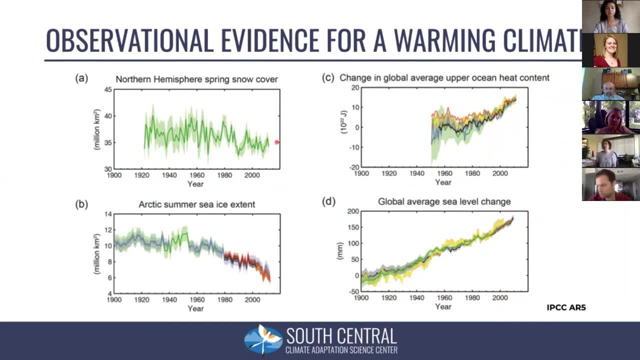 um the northern hemisphere is decreasing um the upper ocean heat content is increasing. we're losing significant amount of sea ice in the arctic and uh we can measure the rise in um a sea level as a result of glaciers on land melting and adding that water in into the big. 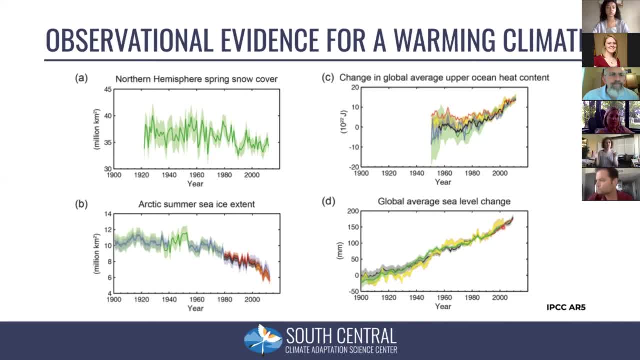 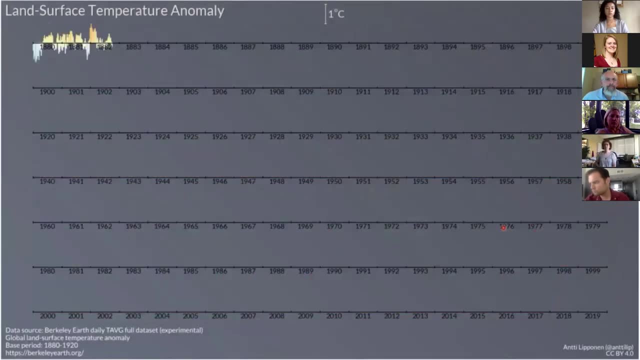 ocean buckets, um, but also in those ocean buckets, uh, water expands when it's warm. so even without adding that extra water, we get sea level rise, and so, uh, we can also then look at our changes in our temperature over time. so this is a record from the late 1800s, averaged over land. so 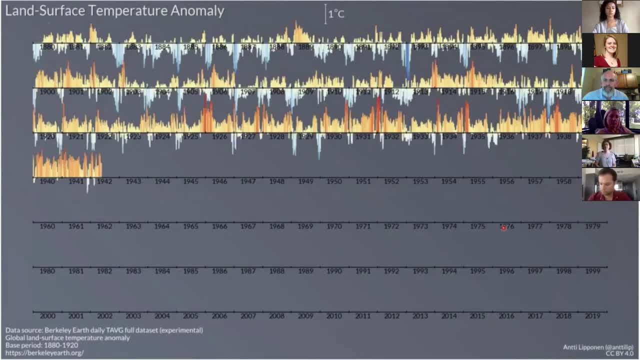 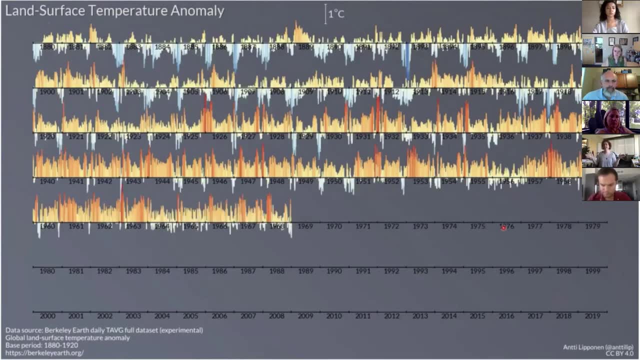 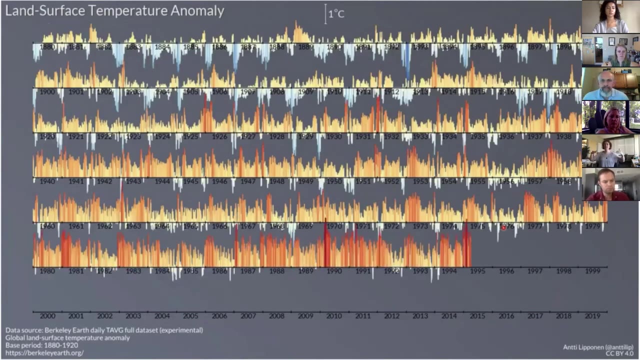 at weather stations, um, and this isn't on. this is the anomaly. so so the base period here was from 1880 to 1920. so the black line represents um, uh, that period of time. anything above that is warmer. that month was warmer than um, the base period. anything below that, uh, the earth was cooler, or? 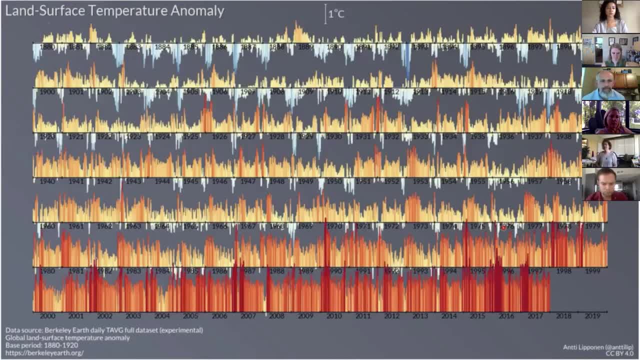 for that month and what we see is that, um again, we see monthly and uh annual changes. so we still see all of our el nino and la nina cycles and our daily uh weather and climate variability. that occurs, but over my lifetime, which goes back to 1980, okay, 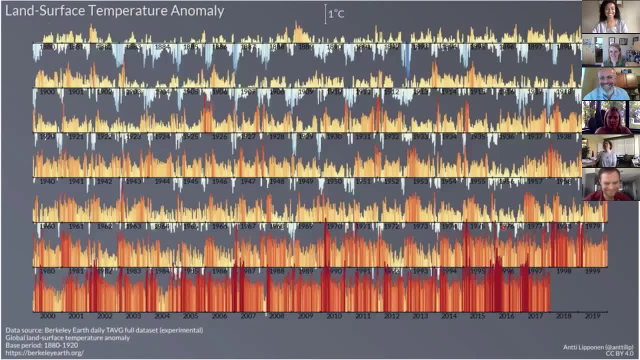 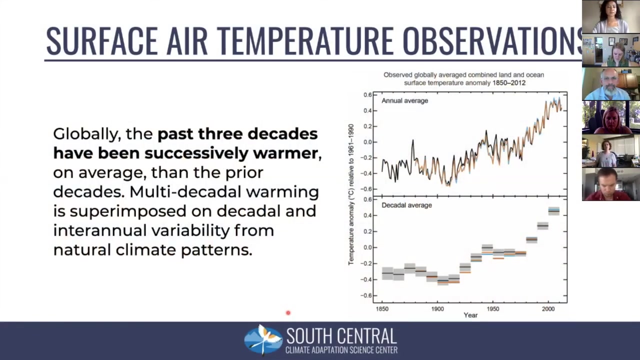 maybe not so believable but um, over the lifetime of all of the college students that i supervise. they have only seen a few months in their lifetime that has been below average temperature. so clearly, especially in the last few decades, we're seeing a significant increase in those surface temperatures. these are globally averaged surface. 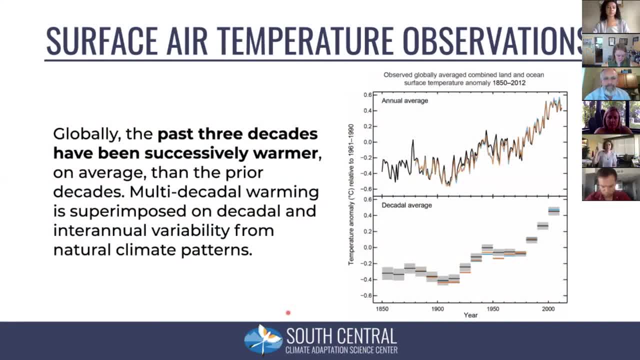 temperatures. so what happens at you, in your state, for a given year is a little tiny blip in the data. even the united states- the united states is three percent of the data, covers three percent of the earth's surface. so even a very frigid or a very warm year in the us is a little blip in all of. 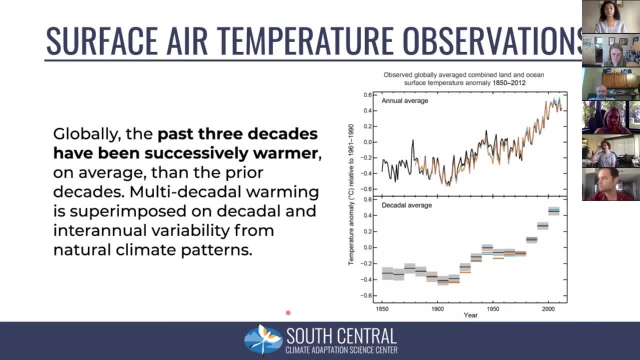 this global data and we can look at this um by decade and you can actually see some of this natural cycle. so this uh cycle here is a result of the atlantic multidecadal oscillation, but superimposed on that natural cycle is this increase in our temperatures. 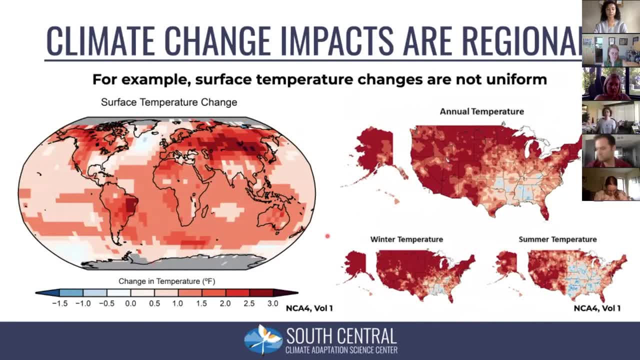 now, even with this globally averaged increase, what you know is where you are. it depends on where you are, on what impact you're going to get, and so the impacts are regional, which is what we're going to be talking about for the rest of the semester, rest of this um uh workshop. those impacts are regional. we see um temperatures in the 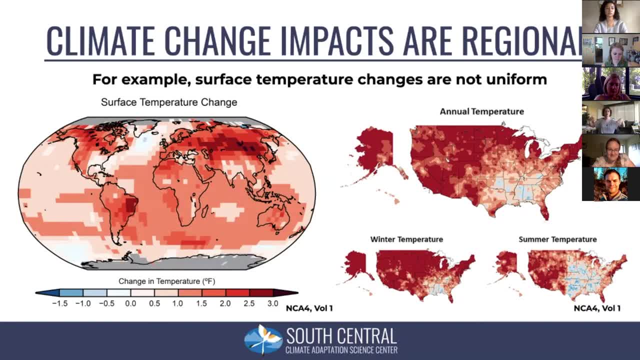 far northern hemisphere are increasing faster than temperatures elsewhere. that's that arctic amplification as a result of um, as a result of the snow and ice melt. but even in the united states we see a region of our united states that over the last 100 years 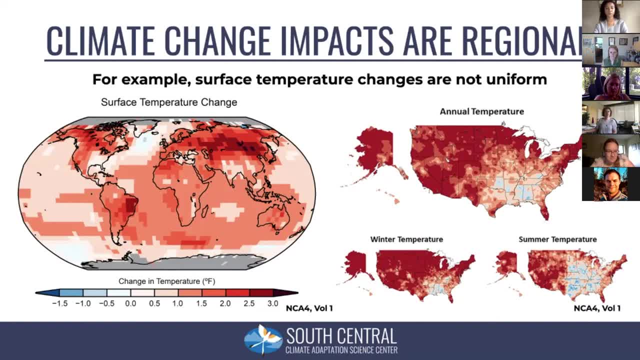 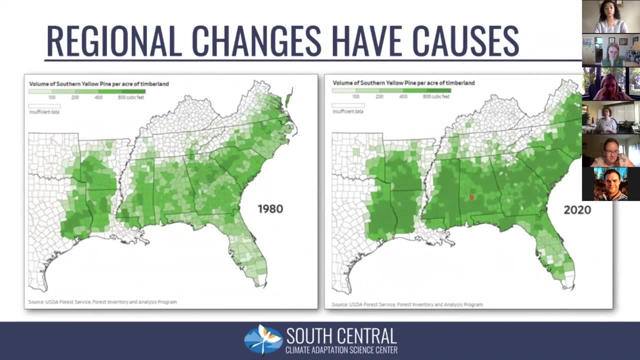 had actually cooled some, and so it's no surprise that many people within our area don't think climate change is happening, because we've actually seen some cooling, and this cooling is um likely a result from the increase in forests over the last hundred years, and that's because Arizona has a 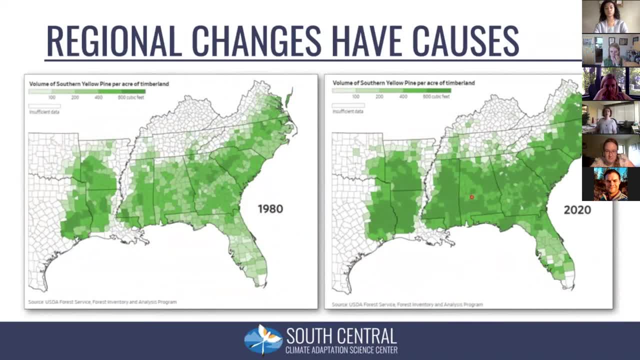 lot of climate change activity that's happening. we've actually seen some cooling and this cooling is um, likely a result from the increase in forests um over the last decade, and so we've seen a significant increase of that and the weather last century in the southeast part of the United States. You add forest, you add transpiration of 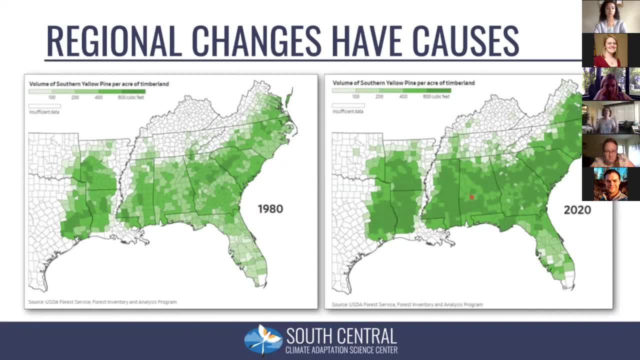 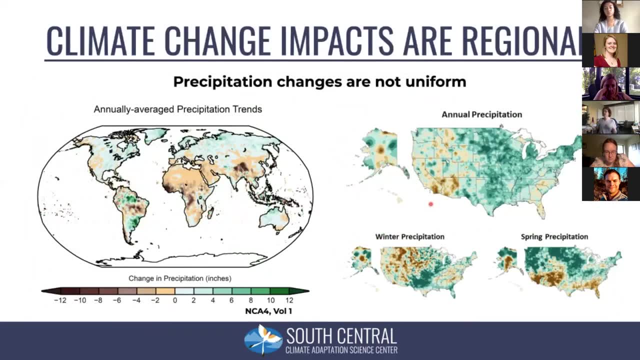 water Transpiration is a cooling process, and so we have some localized land use that's affecting that. Again, things are regional in terms of the precipitation that we see and the changes. It's not only regional, but different precipitation changes will happen in different seasons, so we 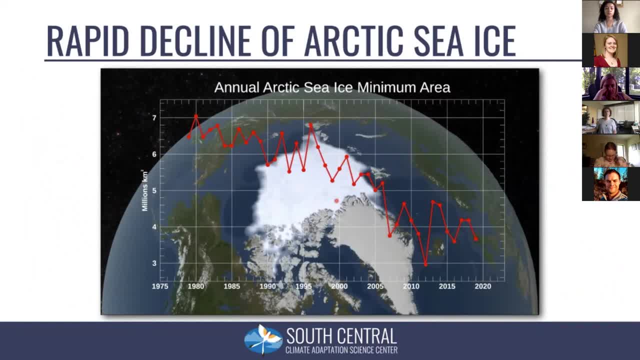 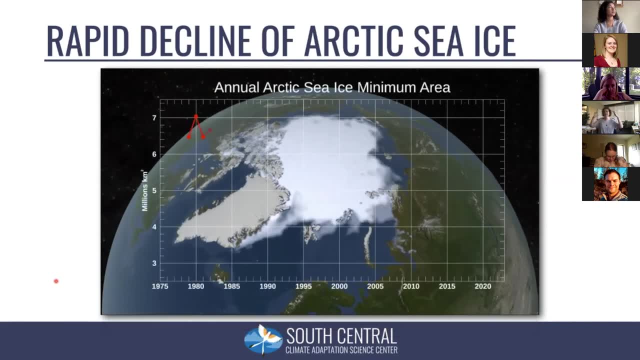 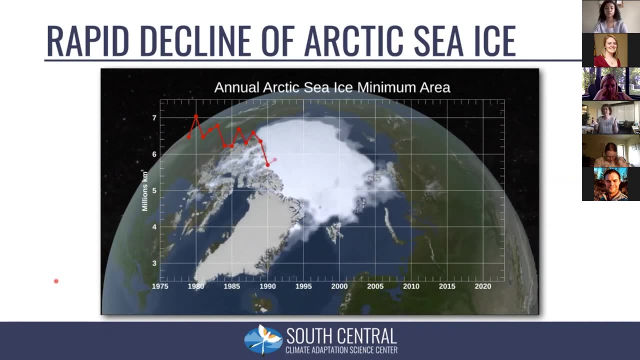 want to keep that in mind. We do see that the ice in the Arctic is declining. so this is the extent of the ice as measured from satellites. so the record isn't as long as some of the records that we have, because we didn't have a satellite until the late 1970s over this region, but not. 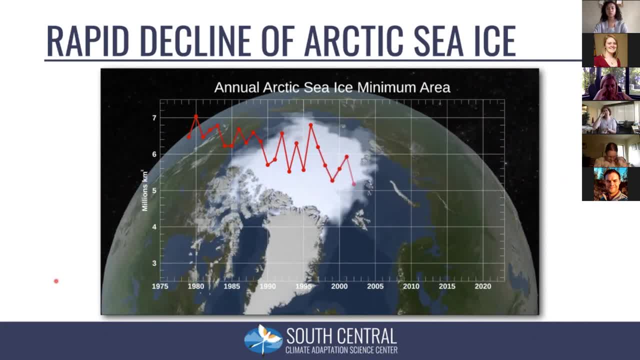 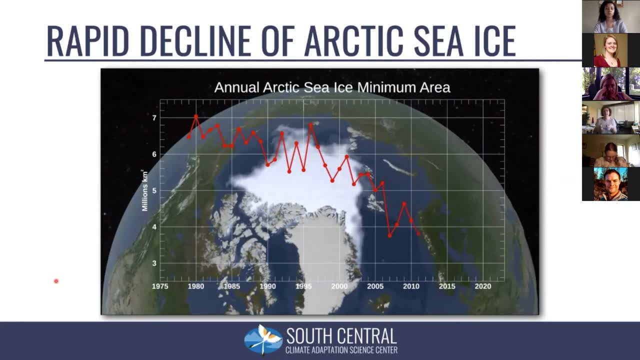 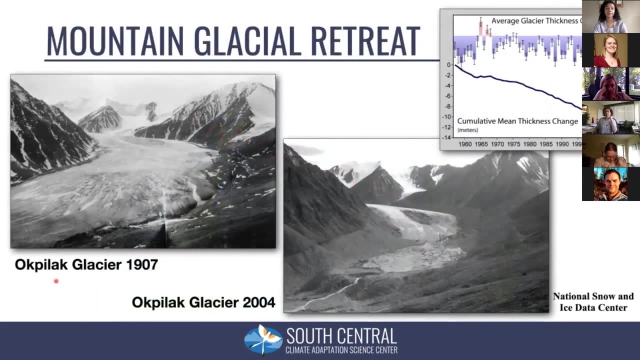 only that, the thickness of that ice is decreasing and the age of the ice, The old ice is being melted- that old, stable ice- and we're getting very young ice. that's occurring. We see similar things happening with the ice on our land. so there are several glaciers across our earth that are increasing in. 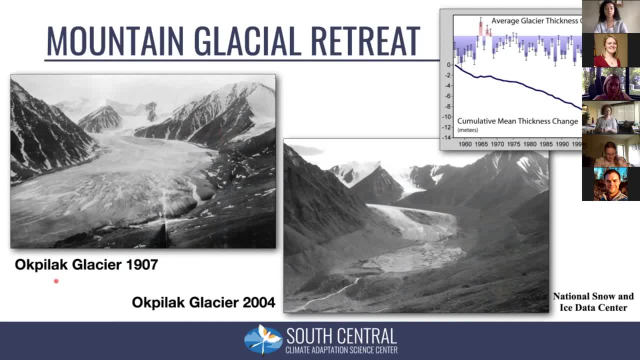 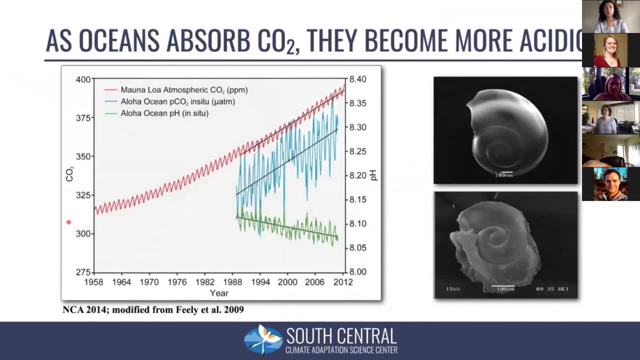 size because of additional precipitation that has occurred as a result of climate change, But most of the glaciers across our earth's surface are decreasing in terms of extent and also thickness. We're seeing, in addition to these increases in carbon dioxide in our atmosphere. we're 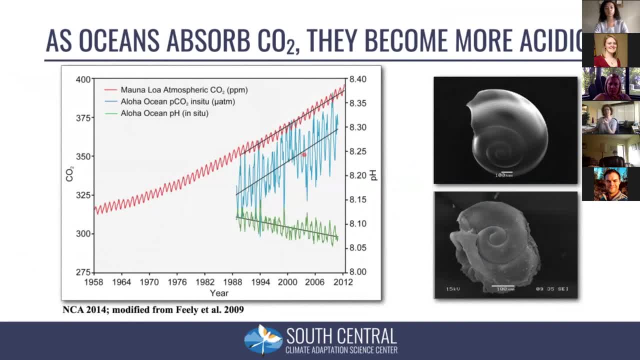 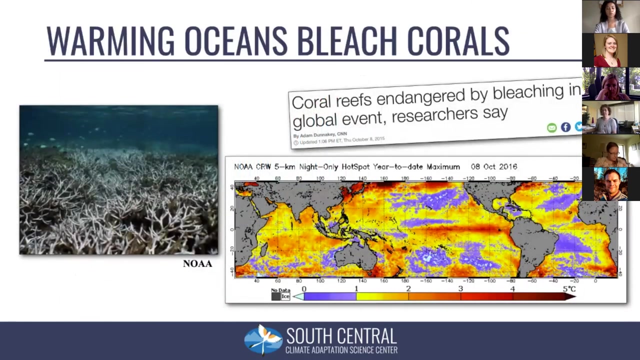 measuring those increases of absorbed carbon dioxide in our surface- ocean surface- and carbon dioxide that's dissolved in water makes that water more acidic, so we're seeing the pH of that water decrease, which is affecting the shells of our sea life. It's also affecting rigid skeletons of coral, but not only is that. 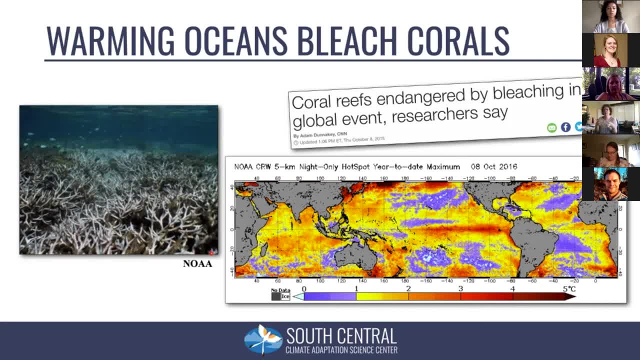 affecting it, but the warming of the waters is actually affecting those corals too. When those waters get warm, the coral gets stretched, stressed, and when the coral is stressed, it releases the little algae that are with them, the colorful algae. 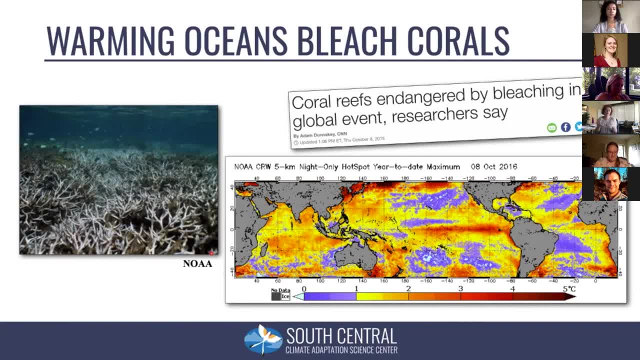 And turns into essentially just that coral skeleton structure and that's usually kind of whitish or gray. and we're seeing these coral bleaching events not only by the asking but also by the density of the coral's life. and so we're seeing these coral bleaching events. 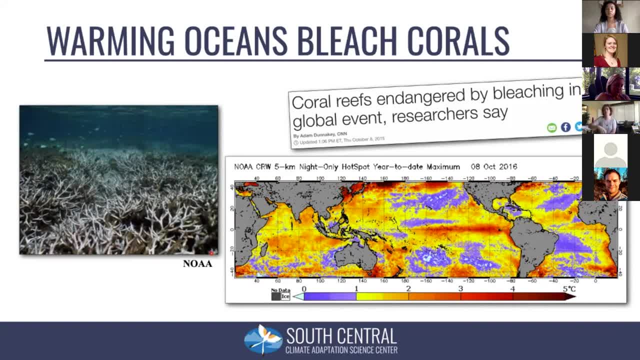 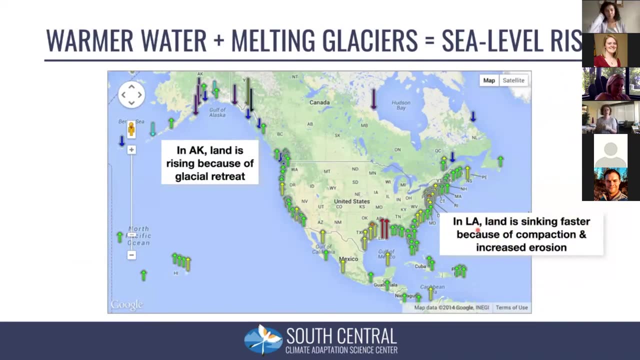 events occur, especially during El Nino events, where those ocean waters get even warmer, So these bleaching events are occurring. We're seeing again sea level rise, but this is regional, So it depends on what the land is doing. in Louisiana, along Texas coastline, We have subsidence. 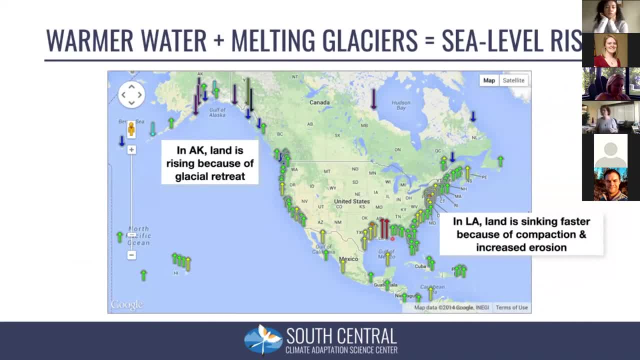 of the land as a result of a number of human-caused compaction, So that's superimposed on sea level rise. So the Louisiana Delta is kind of the poster child of sea level rise in the United States, Whereas in Alaska where we're removing weight of that ice from those glaciers. 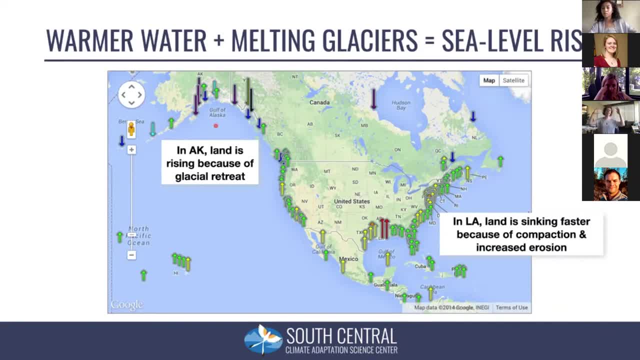 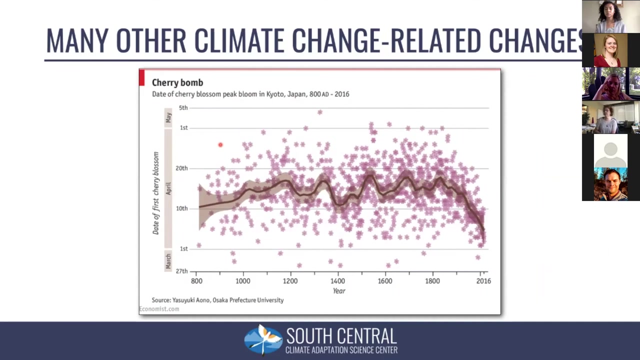 on Alaska, the land is rising up because of the geology that a whole bunch of you know. it rises up in the asthenosphere as that land gets lighter, and so we're actually seeing some sea level falls. we also have changes. there'll be a lot of changes that will be discussed in the next two days, but 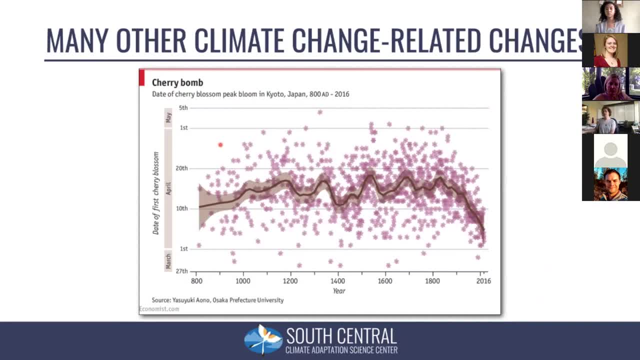 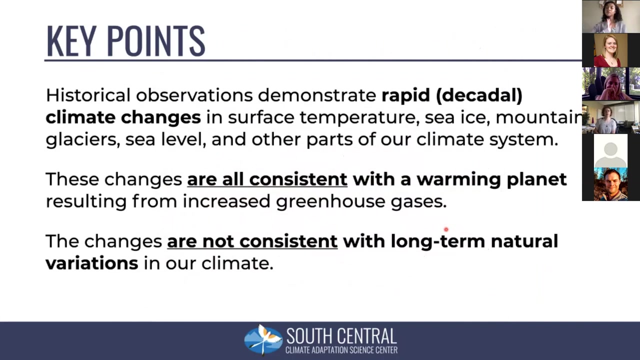 here's kind of a lead-in to some of the changes that we're seeing in nature. this is an example from Kyoto, Japan, where they looked at the peak of the cherry blossom, and we can see in just the last few decades that that's getting earlier and earlier in in the year. so we're seeing what in. 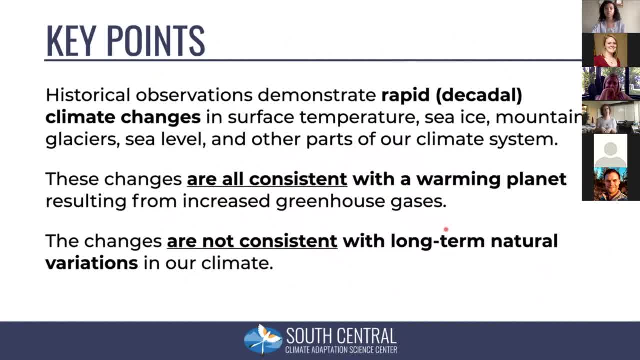 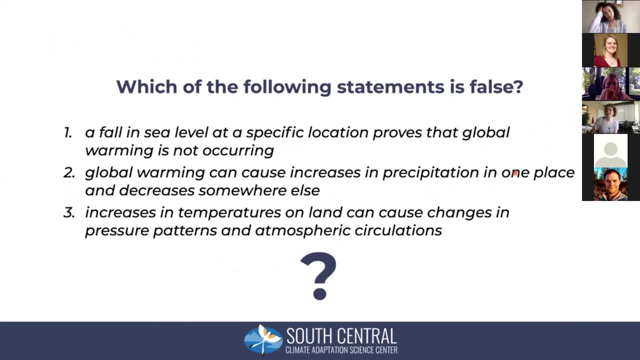 the climate world we call rapid changes. these are on a decade level. these are changes that are affecting the entire natural system. these are all consistent with a warming planet and they're not consistent with just long-term natural variations. so the last question that I leave you is looking for the false statement here. 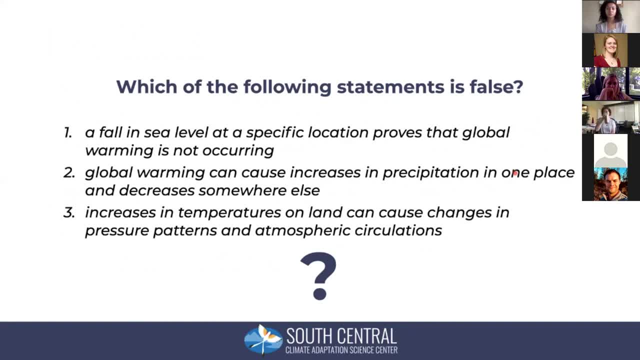 but I'm going to leave it blank because I know it's a good question for me. I don't know if you can see it, but I've got it down here, so I'm going to leave it blank because I know it's a good question for me. 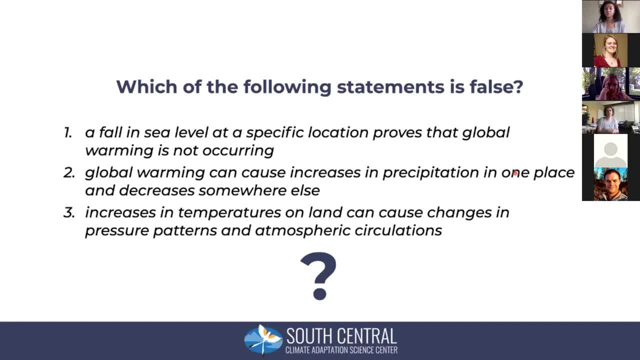 and one of the reasons I put this in is because on Twitter and Facebook and from your family and friends and all of that, you hear things like: but didn't you hear such-and-such, a glacier is increasing, so there can't, it can't be climate change.